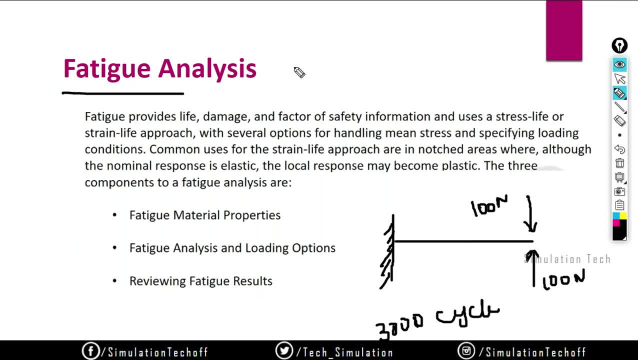 Okay, so what fatigue analysis provide us? like life damage, you can also find the factor of safety information. So, which is related to our component, It's not a separate analysis, it's a plugin of a static structural. first we have to do a transient or a static one, And then you can include the fatigue tool to view the life and damage and factor of safety. So, basically, a lot and lot of theories is actually based on that. 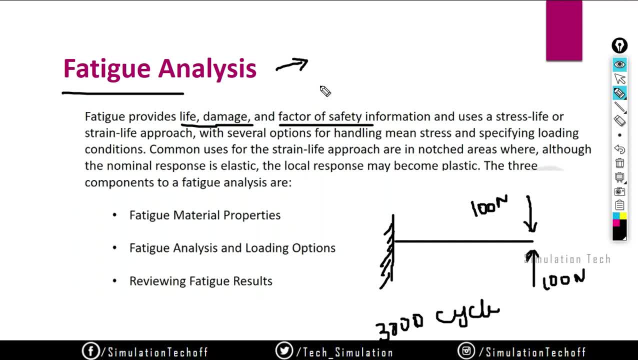 And then you can include the fatigue tool to view the life and damage and factor of safety. So basically, a lot and lot of theories is actually based on that. Okay, so we can consider it as one cycle is like this: So maybe a positive cycle, So half of the positive cycle and half of the negative cycle, we consider it as one cycle. 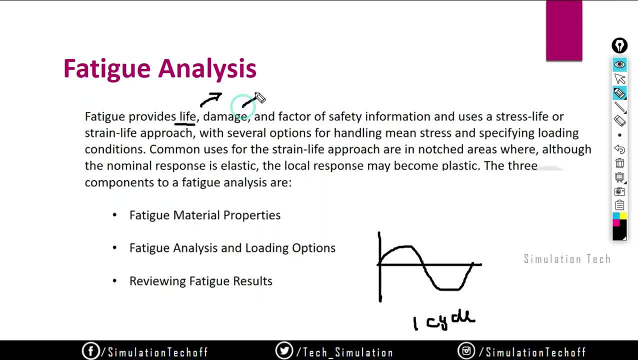 Okay, so we can consider it as one cycle. And what about that damage? Basically, if you get the damage value which is more than one, more than one, your component is surely failure. I mean failed, But you have. if you are getting the value which is less than one, your component is sustainable. 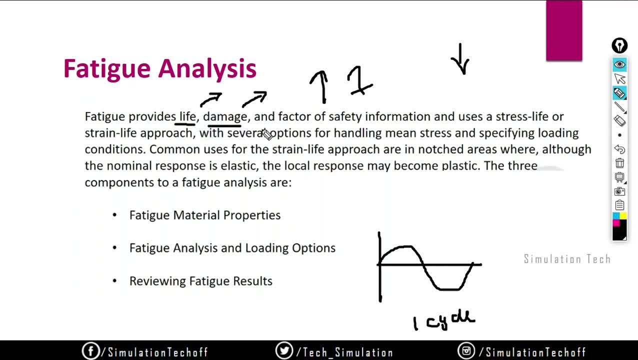 okay, so we will discuss about this terms in software itself and factor of safety it also which is related to the life and damage. the factor of safety can be calculated by using two different methods. one is stress life method and another one is strain level approach. these fatigue analysis is actually carried out, but by these two methods, like stress life method. 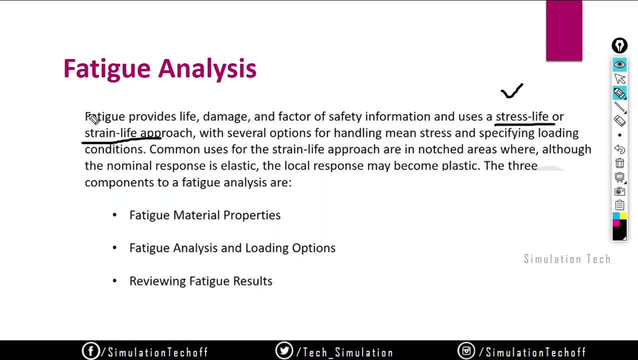 and strain life approach either. you can choose this. it's depend upon our cases. I will explain so. when to use a stress life method and when to use strain life method, okay, okay, basically, the fatigue can be classified into two types: high cycle fatigue and low cycle fatigue. so what is? 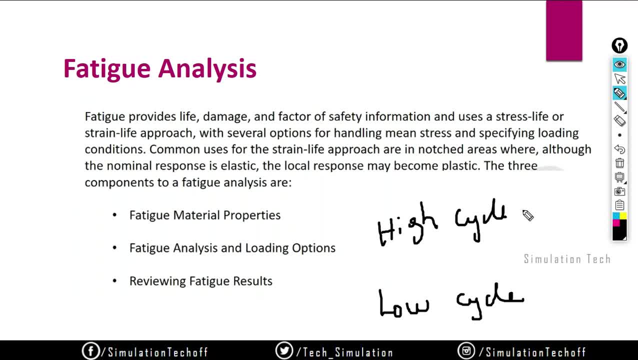 that high cycle fatigue. if suppose my component is not failed, it can be sustained or it can be lost for 100,000 cycles. 100,000 cycles- so I am talking about cycles, not days or whatever it is. 100,000 cycles it is considered as a high cycle fatigue. okay, it can lost a large number of cycles. but if your component 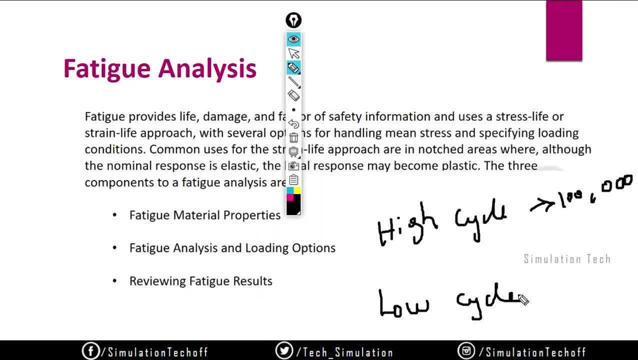 is failed less than 100,000 cycles, it can be lost for 100,000 cycles. so if suppose my component is failed less than 100,000 cycles, it can be considered as a low cycle fatigue. so only you can classify by this method like either it should be a high cycle or it should be a low cycle fatigue. okay, so 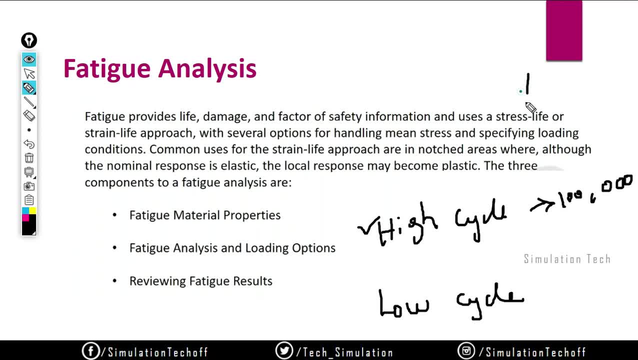 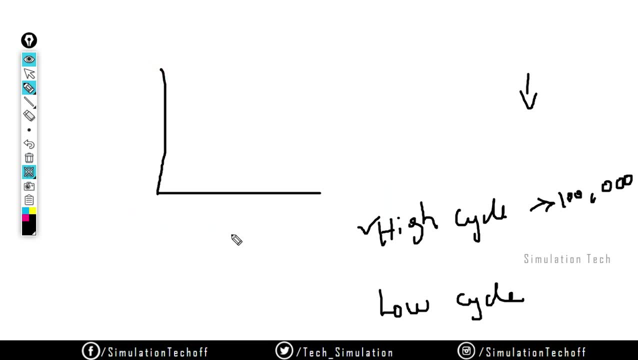 if it is a high cycle fatigue you can go for the stress life method. basically, a high cycle fatigue component is actually failed in the elastic limit. so I hope you know that what is elastic limit? so when I try to draw the SN curve, that is stress versus number of cycles, that is a 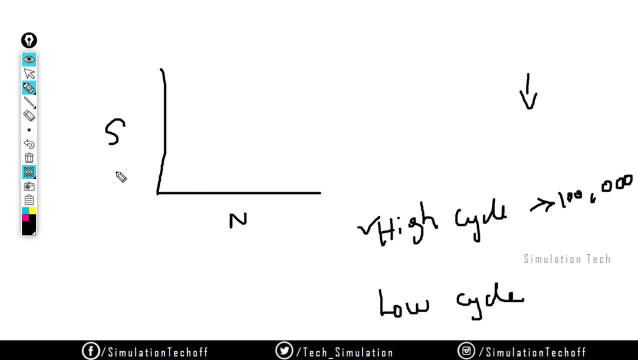 how many numbers it is. actually. you have to convert these curves into a log to 10 plot. I mean log plot table. so basically it is a material property. so you have this code, the engineering data itself. I will see you, I mean I will show you, uh, how the graph is looks like in engineering data and it should be look like this: 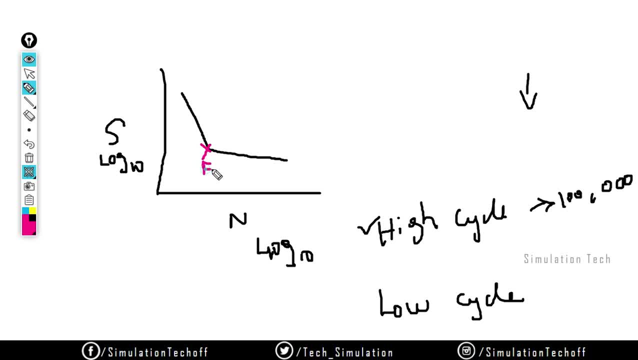 so basically, this is the endurance limit e. So if the failure is up to this point, there won't be any failure. So this is one curve, And if I draw a force versus deflection curve, you are familiar with this curve, So it should be look like this. And if I split this, this is my elastic. 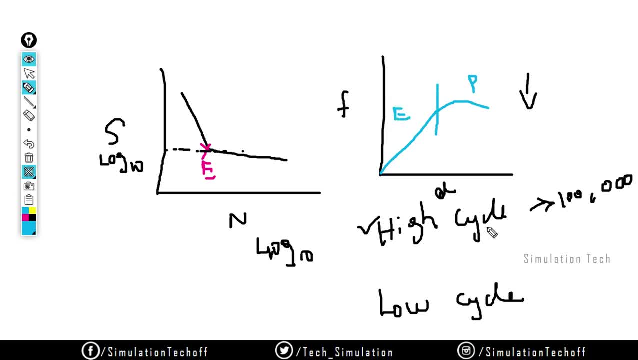 limit And this is my plastic limit. Okay, In high cycle fatigue, the failure is actually happened in the elastic limit. Okay, so we safely ignore these plastic part. Okay, so we've only calculated on the elastic part. If you are using stress life method, the problem 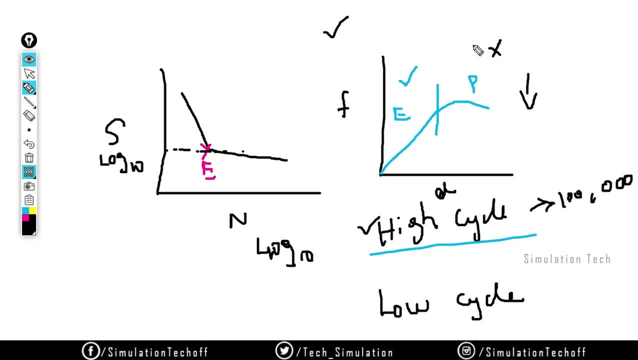 is easily gets solved. Most of the time people only chooses the strain life approaches because it includes the plastic side, also these curvatures, Okay, But for low cycle fatigue we can choose that strain life approaches. Yep, Hope you'll get. 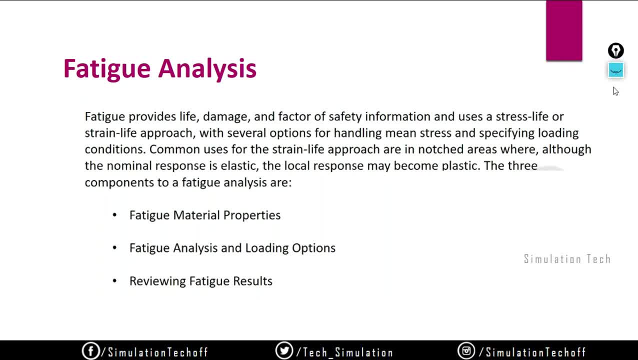 this point And several options for handling that mean stresses. I will explain what is that mean: stress in software itself and specifying the load condition. So basically, we have wide varieties of load defining methods. We have load defining options like these: In fatigue analysis, the load is repeated. 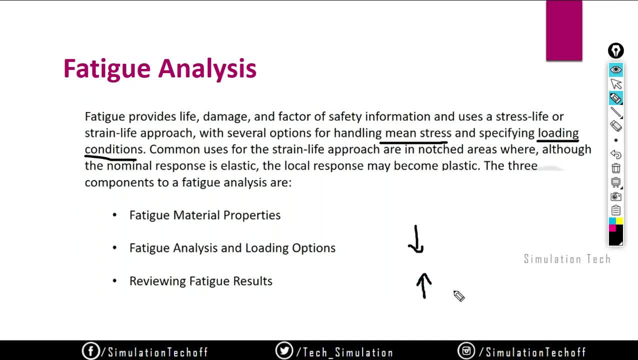 itself right. So one load is in the upper side and another one is in the lower side. constantly it is repeated. We can classify these loads like full method and zero based method has historical data. we will clearly explain this. loading conditions in software. 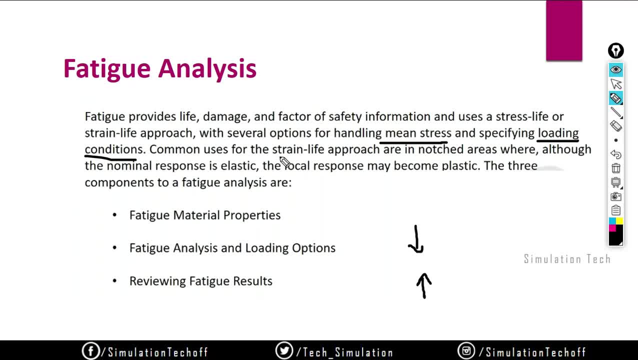 itself. The common uses of the- I mean common uses for the strain life approaches are in the notary areas Where, although the nominal response is elastic, the local response may be plastic. So what they are they are trying to explain here is the strain life method is only for that low. 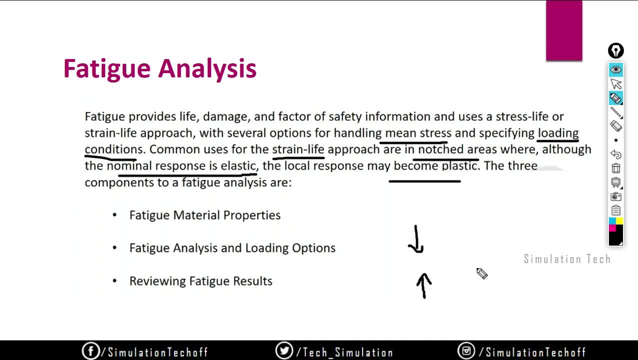 cycle fatigue, that is, having the life which is less than the 100,000 cycles. If your component is clear, so that is no notches or any disturbance in that surfaces. So basically, if you have notches and irregularities in surfaces the fatigue is happened. 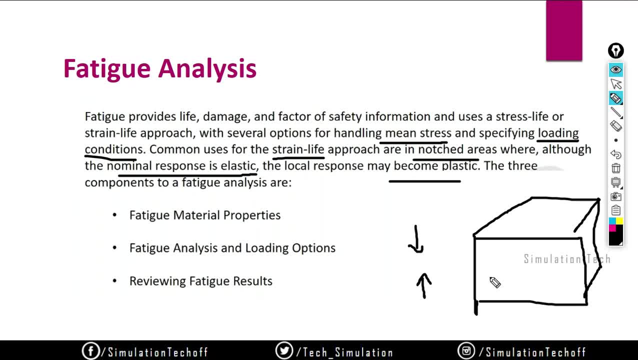 So quickly or so early. Okay so if you have some cracks in that surfaces, so obviously the crack is expanded from the surfaces itself. Okay, so your component is surely failed at the earlier stages. So so the notches areas, these kinds of irregularities, are actually. 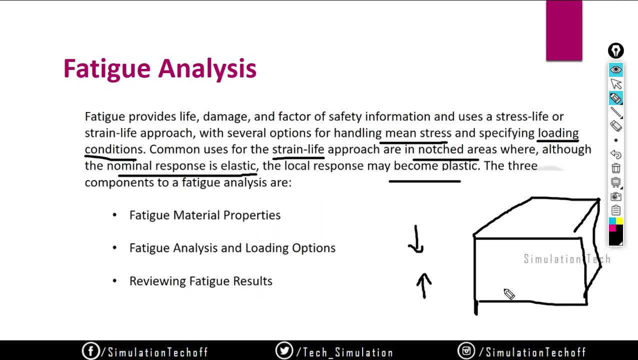 included in the strain life approaches, not included in the stress life approaches. In strain life approaches it actually uses the method called true stress and resistance, The true strain, and you know about, you heard about the stem to stress and true strains. So these are all called that plasticity, the part. we seen this curve right. So this is. 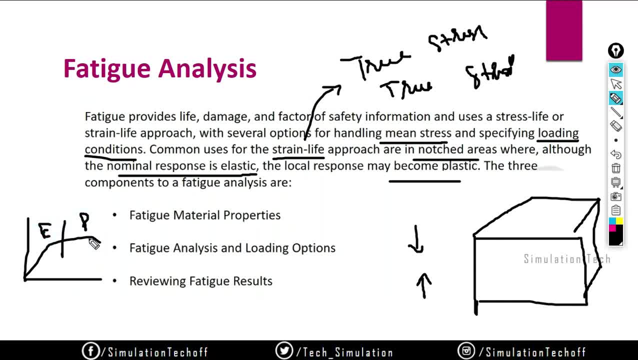 a part and elastic part and this is plastic, these kinds. So these values can be included by using this to stress and true strain. And basically the software uses the curve to calculate some of the factors for the fatigue analysis. for fatigue analysis we need a lot, a lot of factors, values, that is it uses. 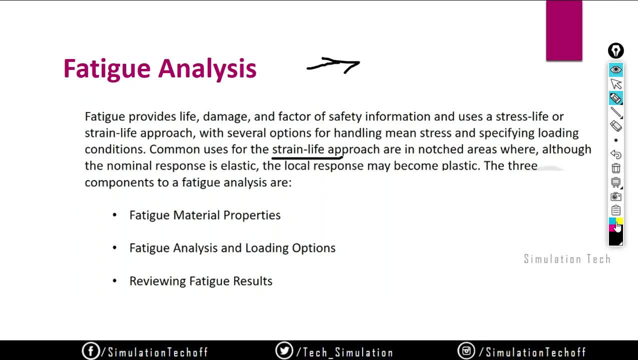 the strain life or stress life approaches to calculate that maybe B1, SF1, and NC1.. So these are all some factors which is needed to cap, I mean solve the fatigue analysis. So these values we can't include at that. 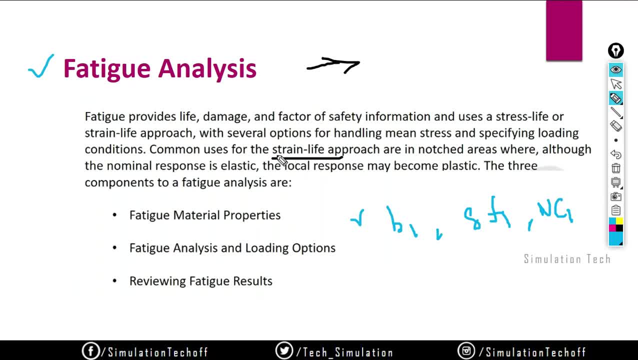 So it can be automatically calculated- I mean calculated from this curves. So stress life method or strain life approaches. Okay, And the three components to fatigue analysis which is very important, that are fatigue material properties. that is, either it may be a stress life curve or a strain life method. 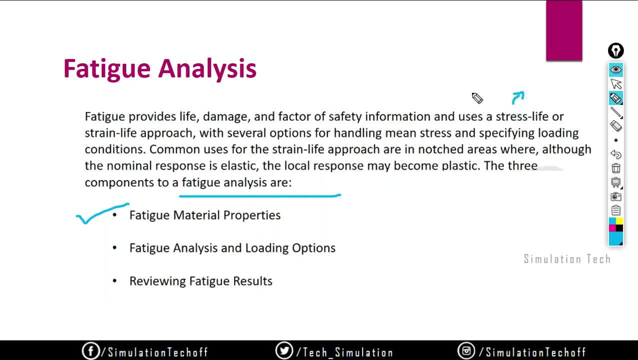 For stress life approaches, we included a curve called alternating stresses, alternating stress curve. Okay, For strain life approach, we include an another curve. So we will see in that And then we are going to talk about, then we're going to study again static pressure. So take. 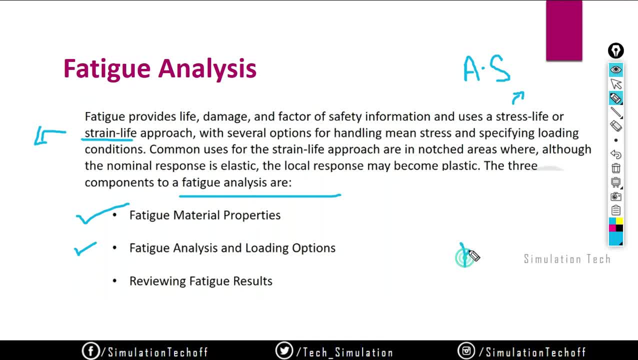 a look at the pattern window, your data in your eyes. we are going to conclude by configuring massDetain Error. We can change the value and loading options. like I said before, whether it is a fully defined or zero based- we have to define that, so that is very important- and reviewing the fatigue result, that is, life damage and factor. 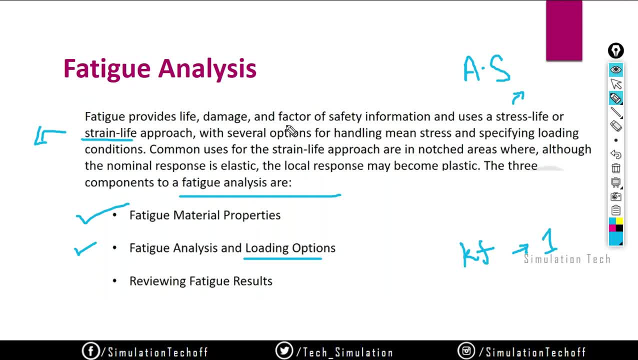 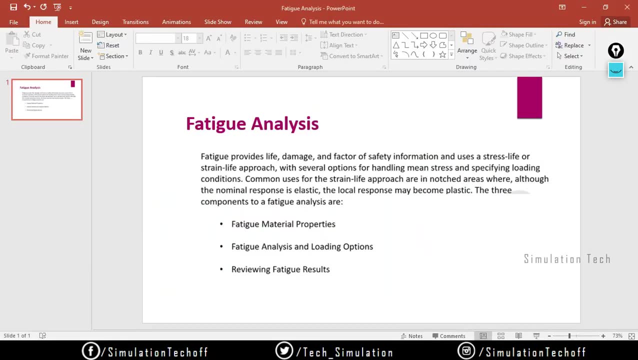 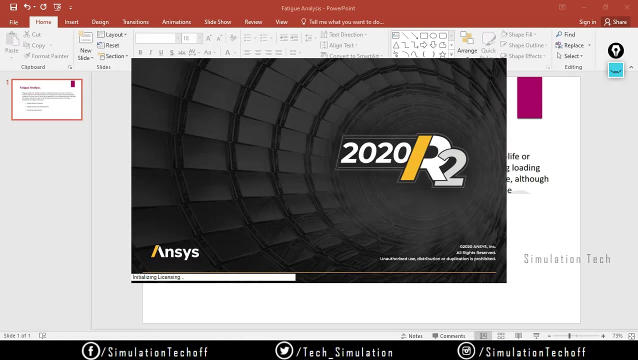 of safety. how can I evaluate so? how can I view the life and damage and factor of safety in software itself? okay, so that is all about the theory session and the remaining will be we will explain in the software itself. so first I will open the workbench, so in the meanwhile I just 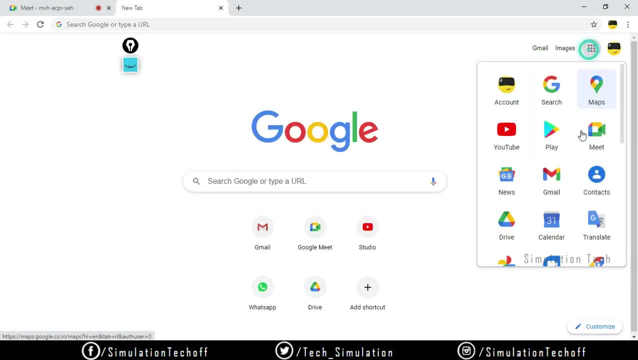 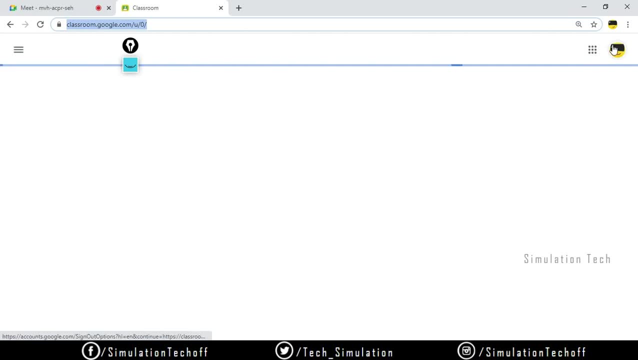 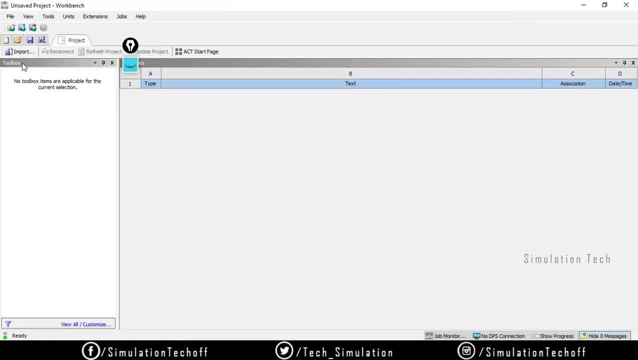 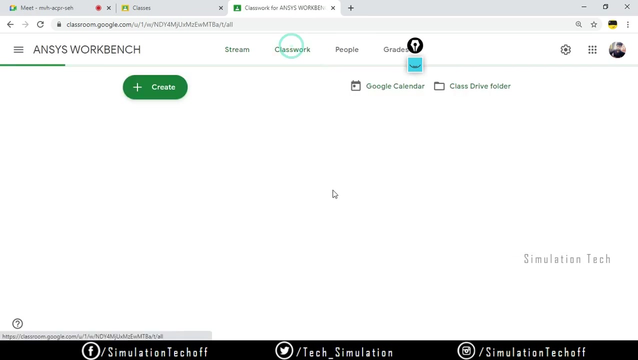 open our Google classroom. this is what I get, but I will skip all the related sections because I will show what that actually is after this. okay, gon. preferences changes in box of Idol to make it work. it is very different, so it is not going to be very deep a lot for me, just using this relations checkbox without. it not, unlike any other program, actually- or browser- is way easier, say not hard enough, because it is ultimcan do the Business ones. this is our 들어가 and it is pretty easy to run desktop apps kind of like jeżeli, video, TwG and simple, but the software will automatically skip. just because the� I, i skip it. it is very easy to run some Plchera by. 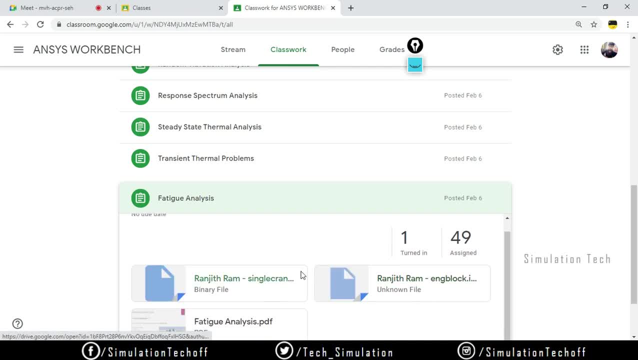 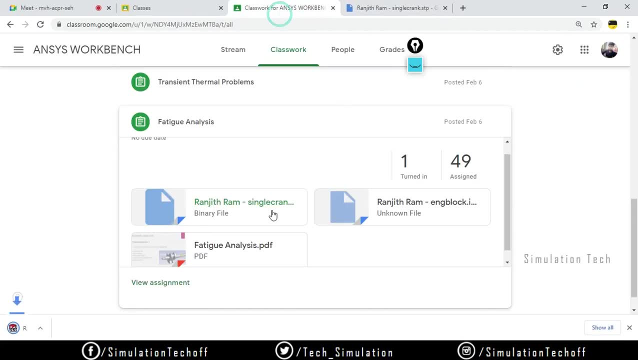 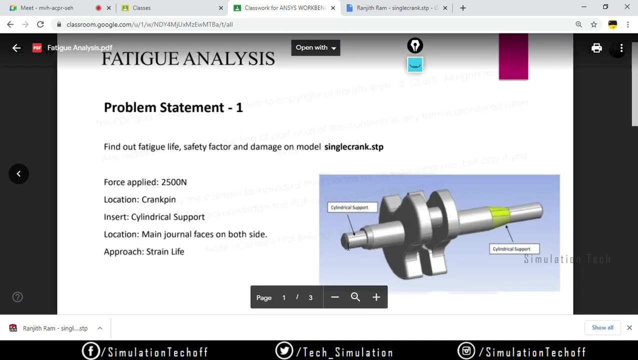 have one fatigue analysis. i will download any one of the model like this crankshaft and also i will open this pdf. so here we have that: boundary conditions. it's very simple to do this analysis. so all we need to do here is we need to find the life and factor of safety and damage on this model. 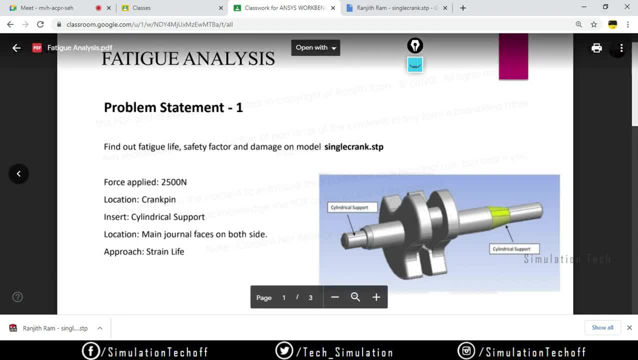 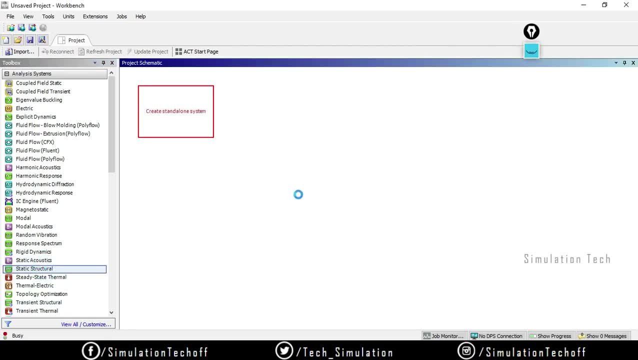 whole. all of this is logical. so again, first i will drag and drop the static structural. so why i actually uh drag and drop the static structure means for fitting analysis. we need stress values, so stresses must. to find the stress, we use the pre-stורה. 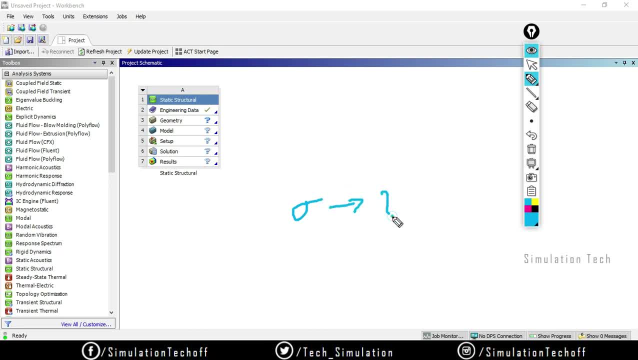 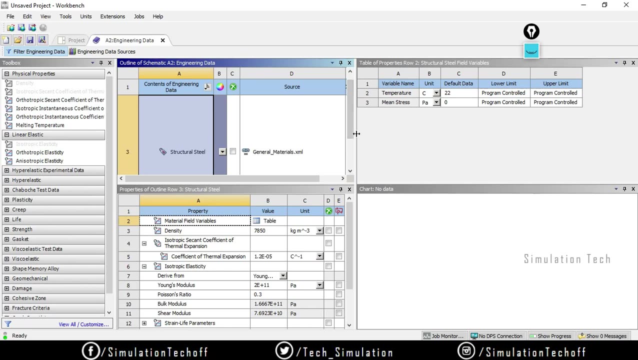 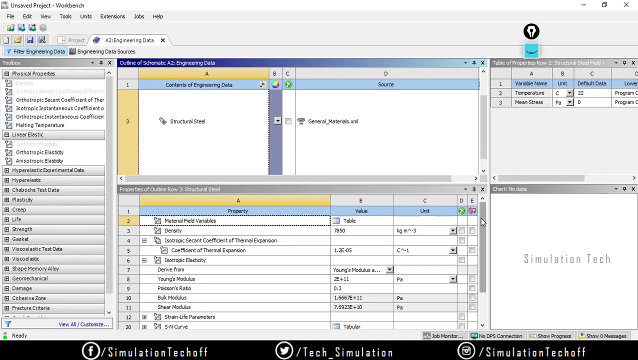 condition that is static, structural, for our analysis. after finding the stresses, we can use uh, uh we, we use the stress, calculate the fatigue properties of this component, and so double click on the engineering data. right now, structural steel is actually added by default. you can check will have two curves, that is. 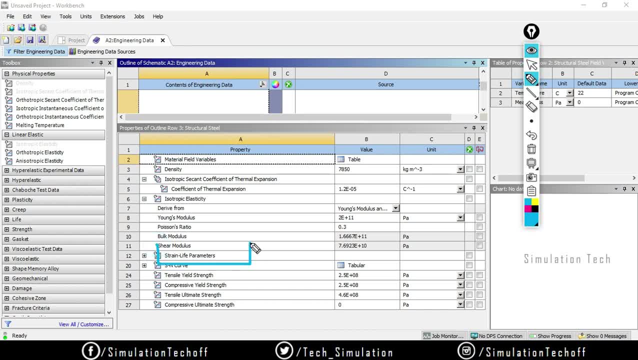 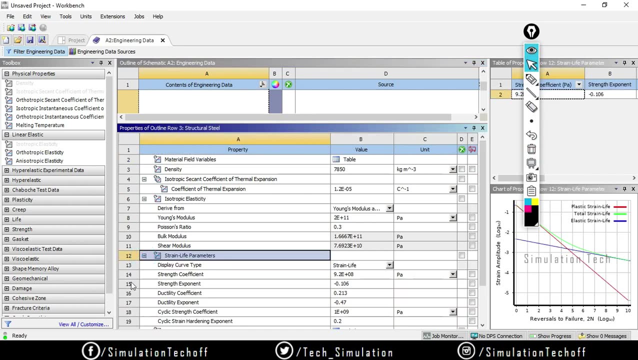 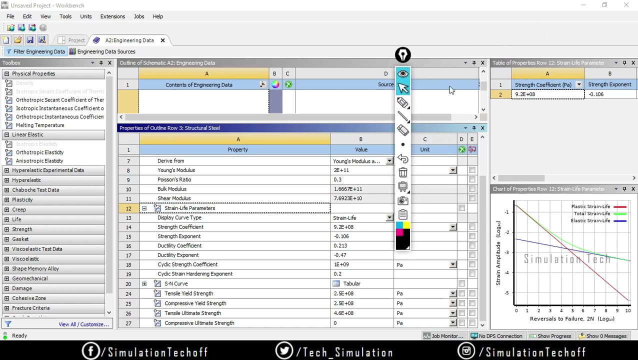 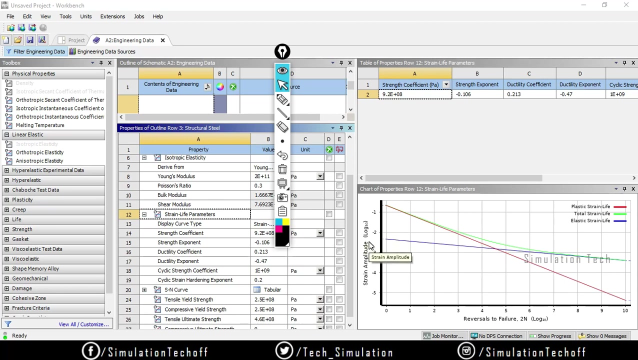 see here. you will notice that these curves stress life parameters and also you will notice that there is an another one that is called sn curve. when i expand these two things and when i click on that stress life method, you will have a curve like this: so, which is actually? uh, strain amplitude, which is logged? uh, uh, log the plot, i'm. 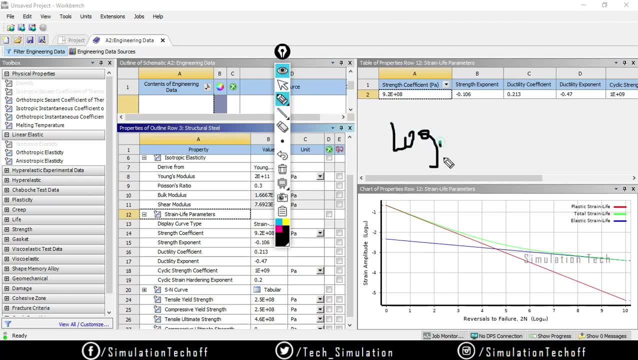 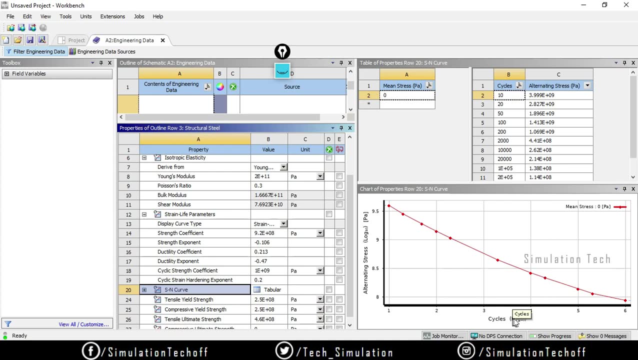 in log10 plot to lock 10 plot. so stress, i mean strain cozero, the reversal of the failure, and also you have an another curve that is uh alternating stress. this is cycles, so this is the endurance limit. so you have a lot of factors. so these curve is actually uh obtained from the experimental method, so it does not uh. 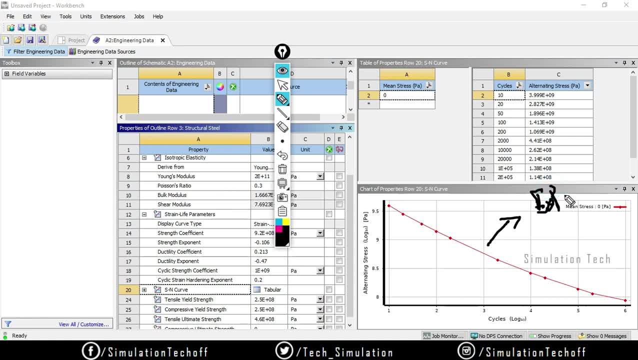 theoretical one, it's an experimental method, yep. so these curves is actually used by the fatigue analysis. so if you are choosing stress life approach, it can use the SN curve, or else, if you are choosing strain life approach, it uses the strain life parameters. and I will close the engineering data right now. I 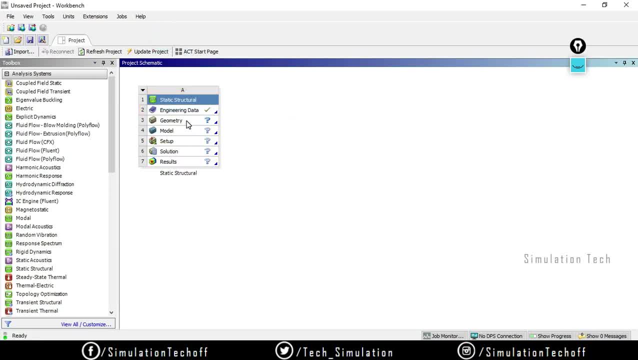 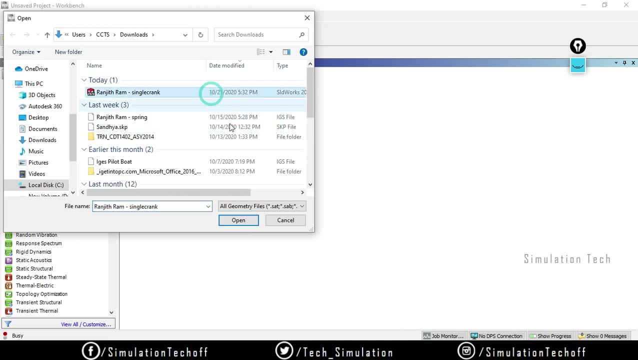 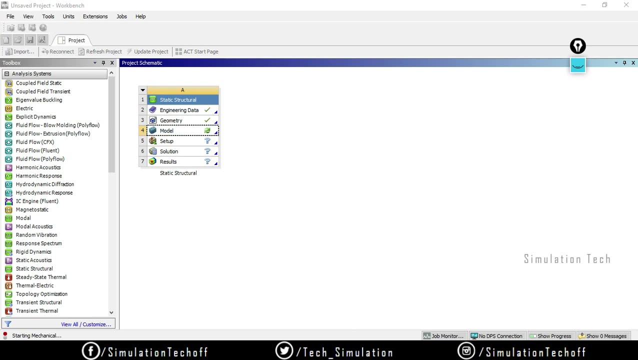 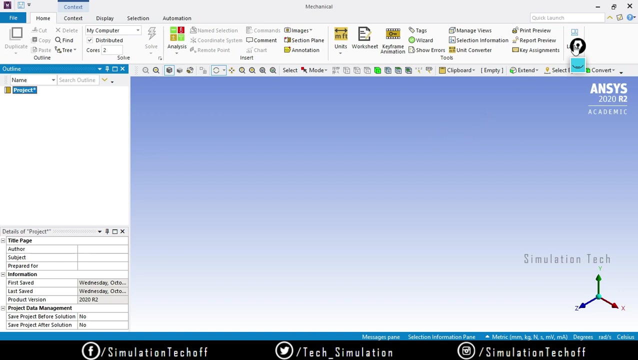 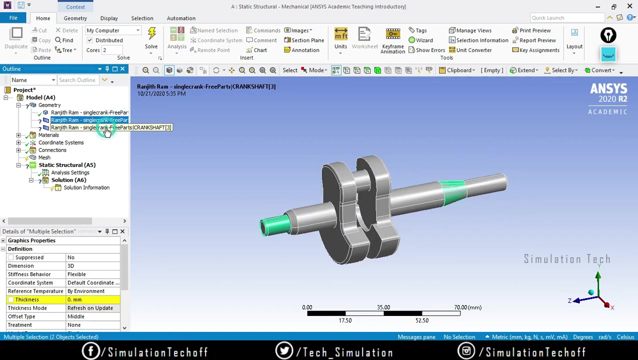 am using structural steel as a default material and I just import the model. I don't want to do any geometry editing directly. go for mechanical itself. okay, so once our model is get opened. so I don't actually needed these two surfaces. what I'm gonna do here is I just suppress the bodies. okay, the next. 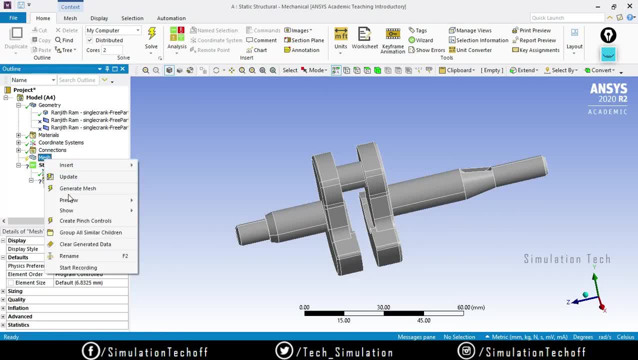 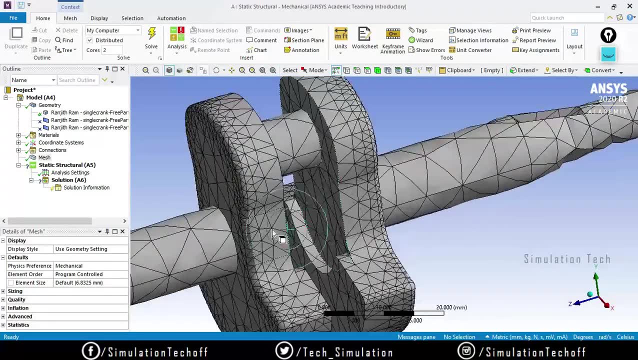 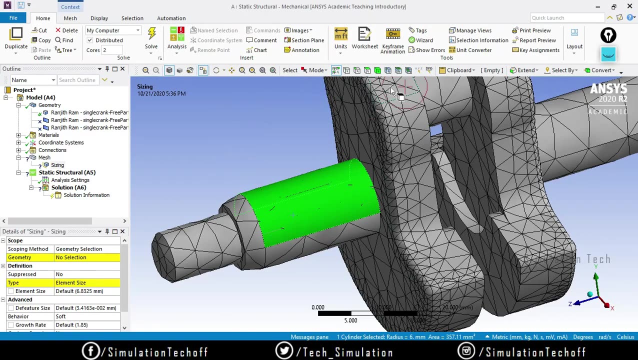 thing is right-click and say generate mesh, so I don't give any factors at all. still, if you want to reduce the size, just right click and see insert sizing. make sure you are on the body selector, select the whole body and click on a plate. you can give the factor. 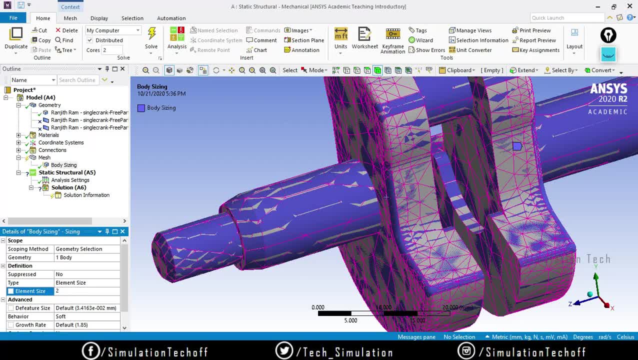 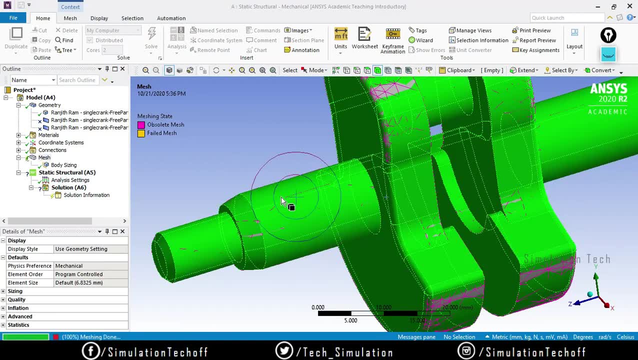 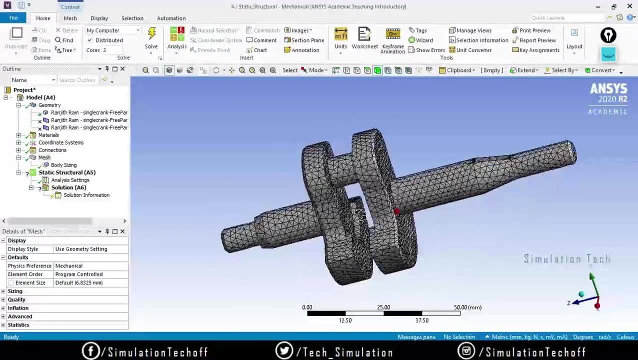 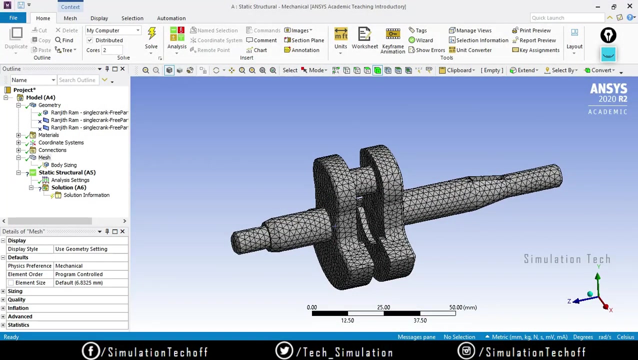 maybe 3 mm. okay, 2 mm is fine. right-click and say generate mesh. and say generate mesh, okay. so now you have a decent mesh. it's not too fine, but it's okay. good, and what is our boundary condition? so we have to apply a cylindrical support and also a cylindrical support over. 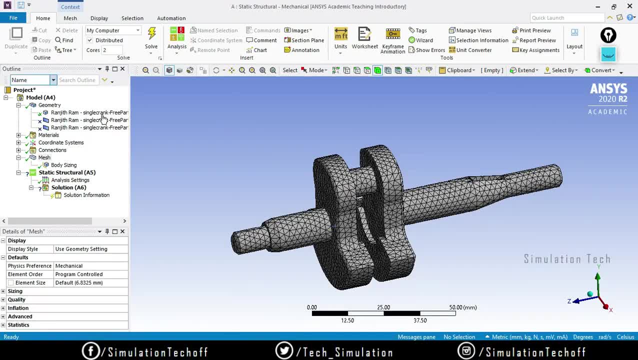 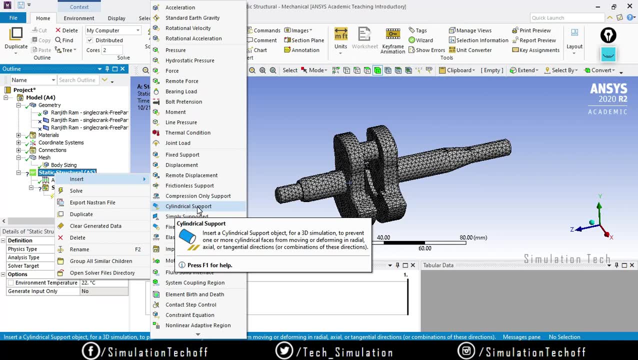 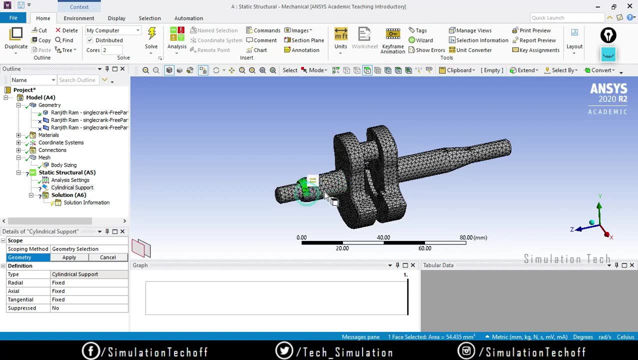 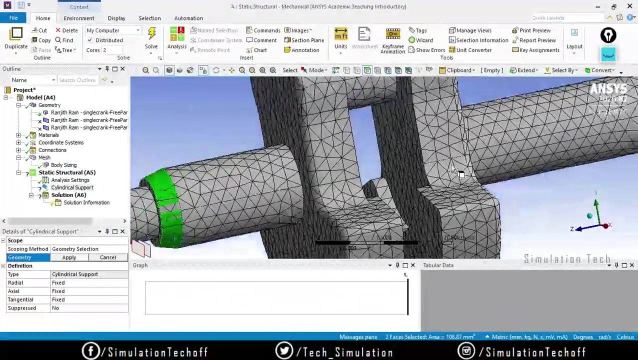 here, but right now I don't want to apply cylindrical support, so you can so right click and insert. you will have an option to apply the cylindrical support itself. so it is only applicable for 3d. so if you want, you can. so just select these and for one side we can. 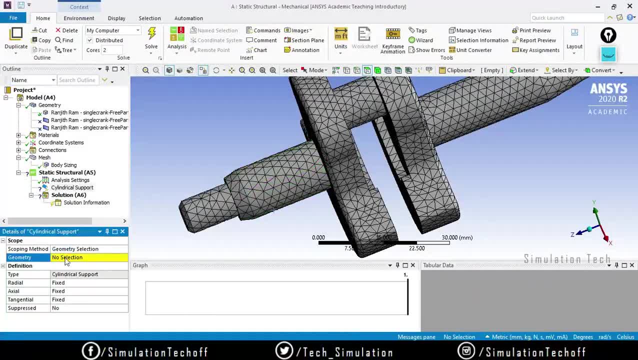 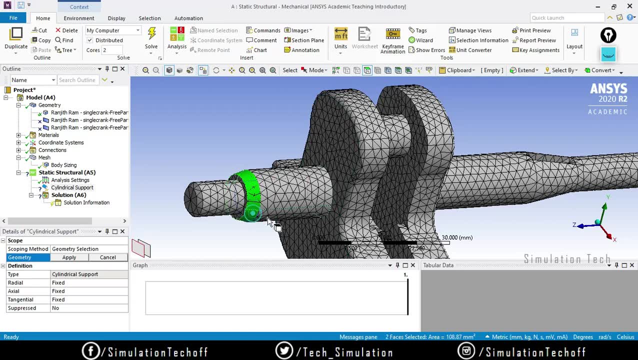 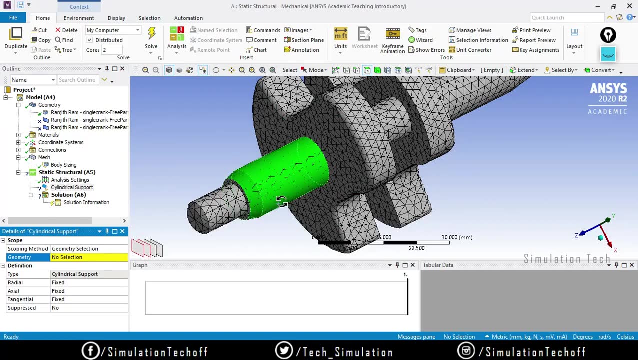 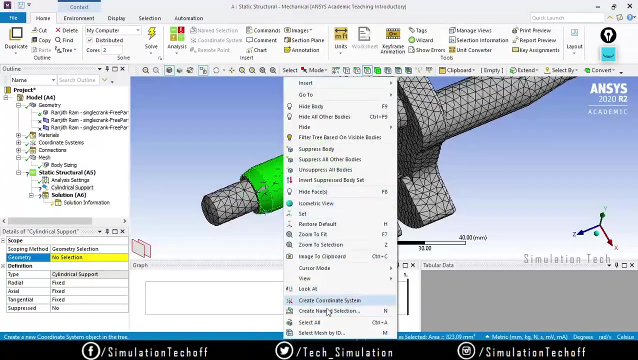 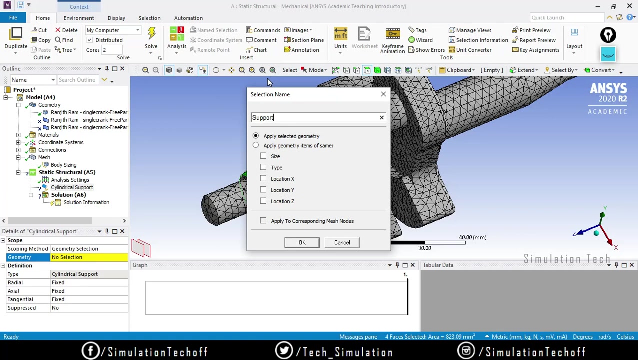 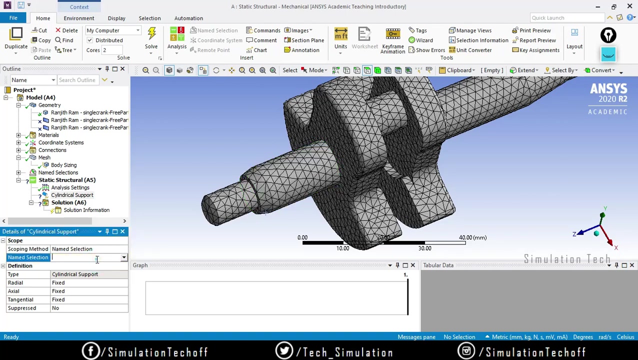 apply a cylindrical support and click on a play and so, if it is not selected, try to create by using named selection- one, two and three. right click and say create named selection support and click on OK and change the geometry selection to named selection. okay, we are facing some issues. 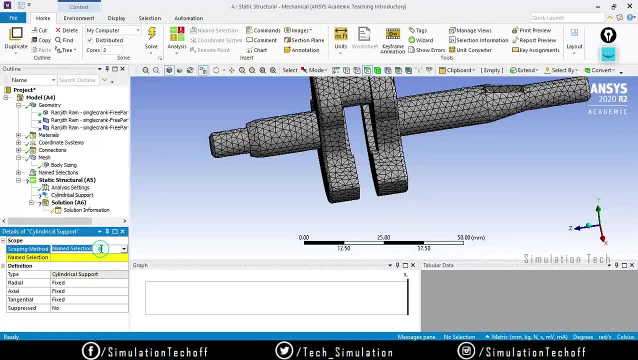 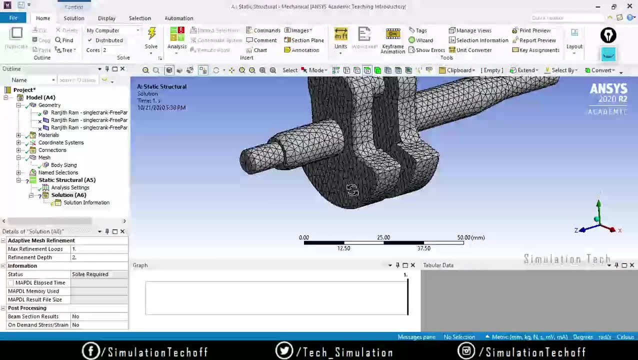 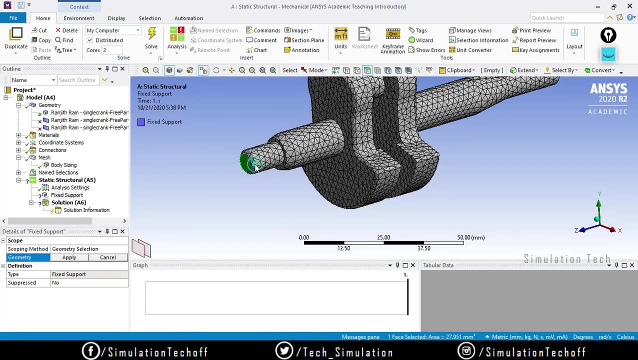 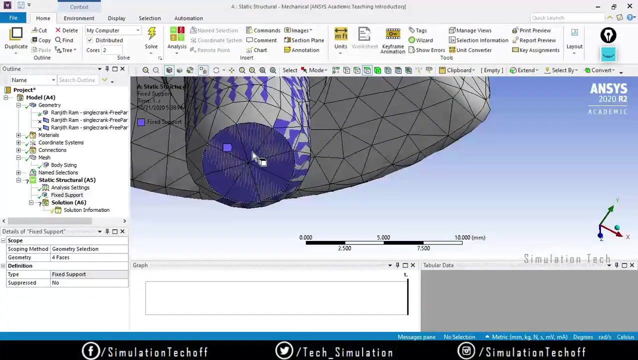 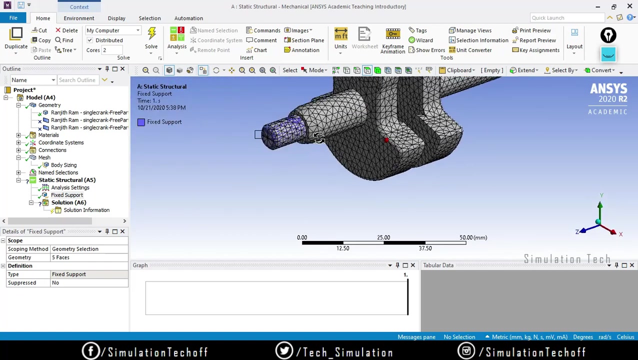 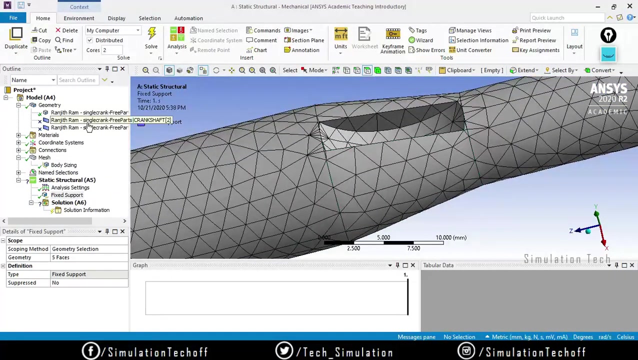 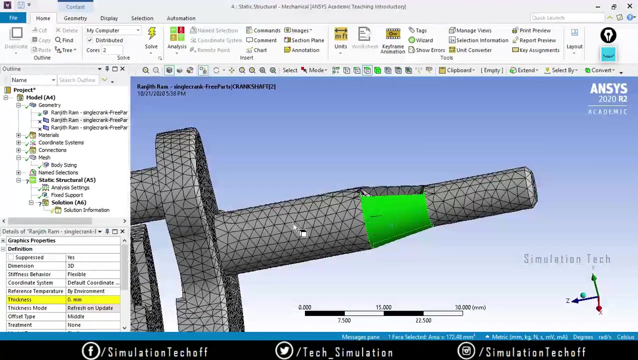 so I'll try to play fix it support, okay, so I want to include these phase also. so I'm going to select this phase and I'm going to also three and click on and click on escapes, and all of five is as a plate. after that I will. 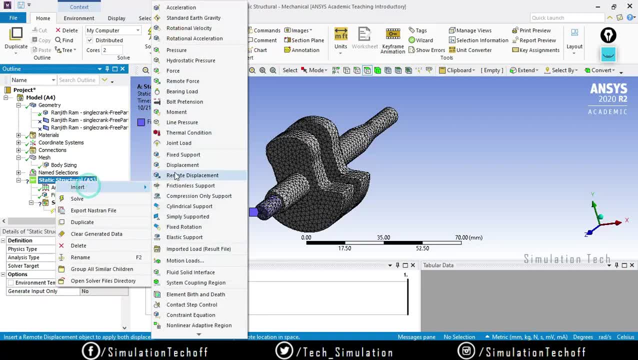 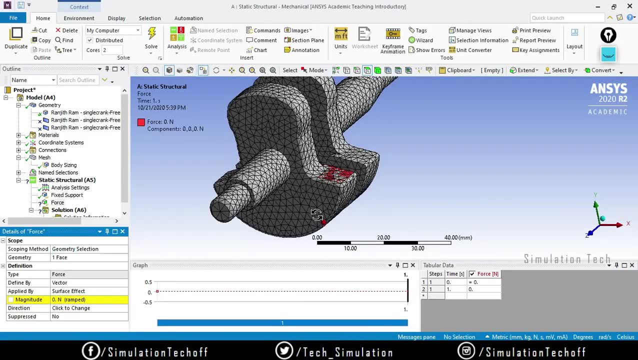 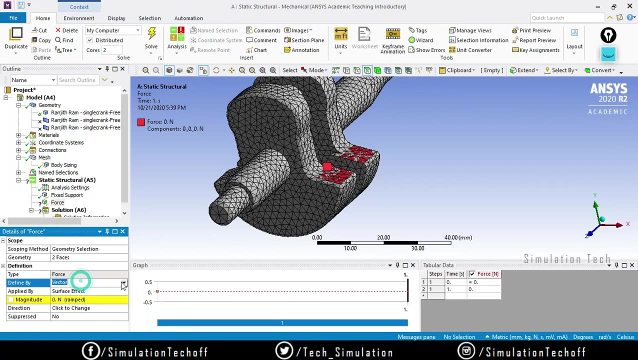 Subtitle now now see c� Audion a pos. this also Subtitle place is a Subtitle, it's completely arbitrary, So there is no case. will also play the space also. And vector two component. so it should be in the negative y axis. Okay, Also, I want to fix this also. 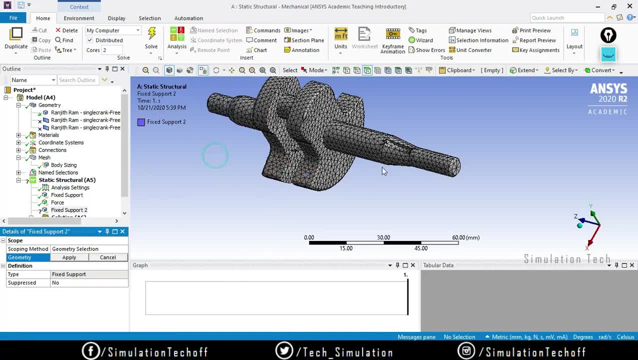 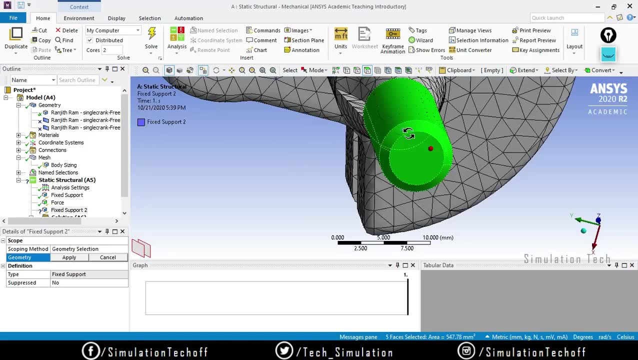 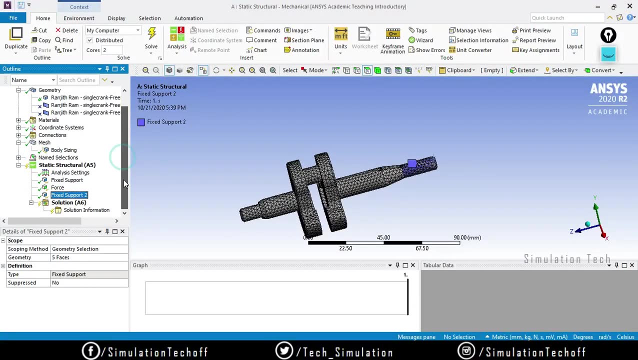 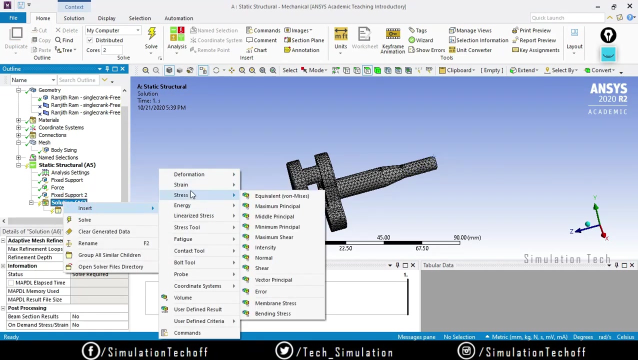 right click, insert, fix it, support. So now everything is assigned. So all we need to do here is: normally we are looking for that deformation and stress results and strength results, right, But today we are going to see about that fatigue. So insert the fatigue. 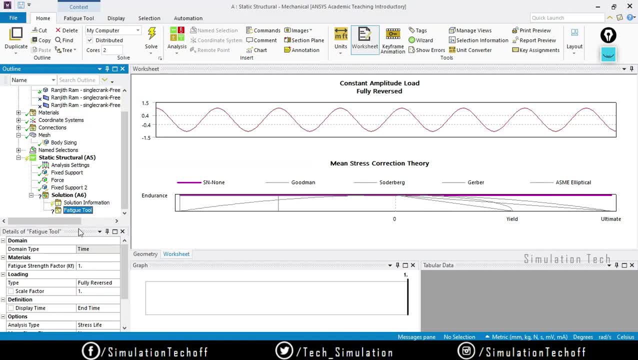 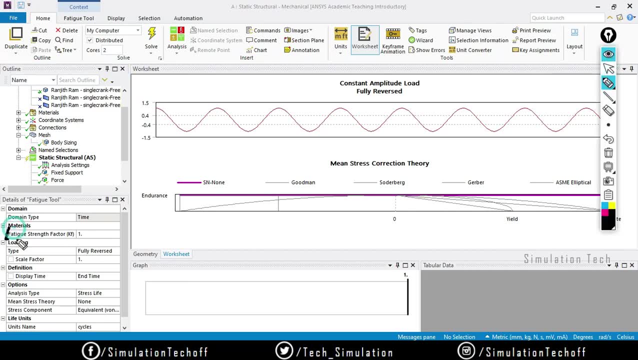 tool. So once you included that, you'll have a lot, a lot of options over here. like K factor First, I have explained in the theory. So these factor includes that whatever the notches or the surface irregularities or your component will go on any quenching process or heat treatment. 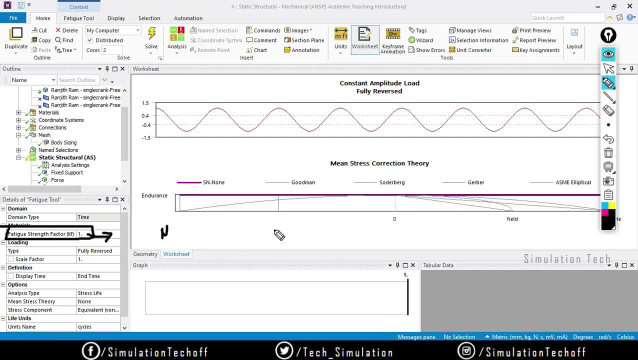 process, If you are having any. I mean doing some additional process like quenching or heat treatment, you may get additional life right So that strength you can include it here by using some factor. So right now software default uses this value, So you can get this. 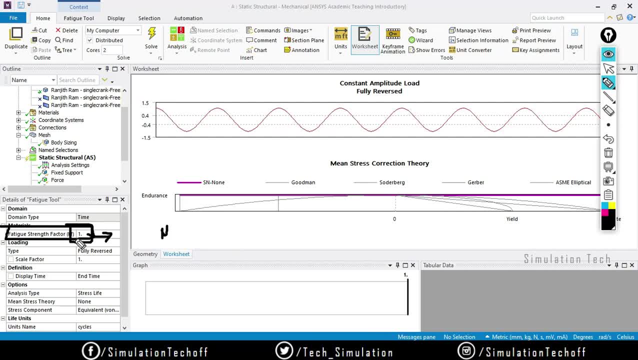 factor in our problem statement, But right now this value is not actually given in our problem statement, Okay, so just know, okay, why we use this factor also. So this factor may increases or decreases, depend upon the- I mean- treatment we do. 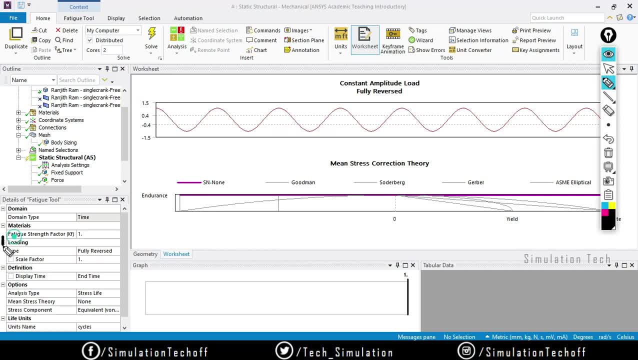 And the next thing is load typing. I mean the loading. So right now it's set to fully reversed. what is means that fully reversed? So when you have a cantilever, if you play 100 Newton of force in this direction and also you apply the same load in the opposite. 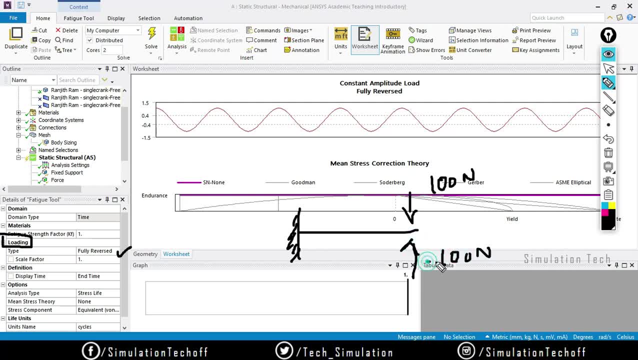 direction, that is, 100 Newton in the negative one. So this case is called a fully reversed one. you will notice that. So from the 1.1 and minus 1.1, it is actually fully reversed. the load is what happened if I change that load typing. 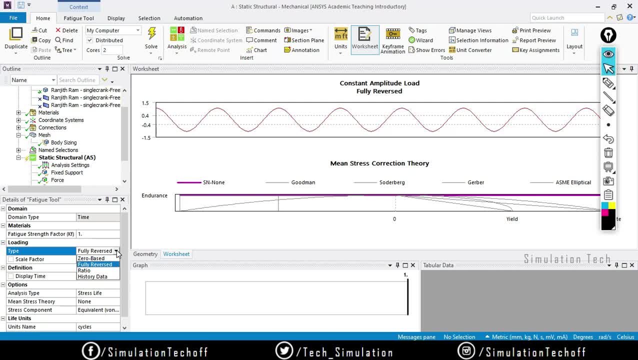 to fully reverse due to. so you have four different types. So zero based, fully reversed ratio and historical data. If I say zero based, it actually apply a reverse load, but return it is not exactly 100, it is 50 or something like that. So from here it is 100. But it. 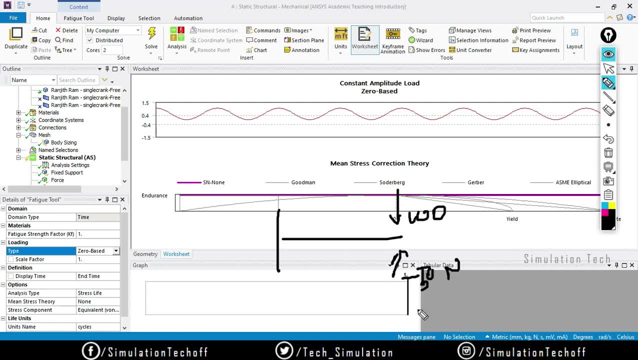 is not exactly reverse the fully load, So it only reverse a partial load. So you will get a partial curve like this, Although in fully reversed the load is actually equal right 100 Newton and minus 100 Newton. If I am taking the mean value, that is mean value. 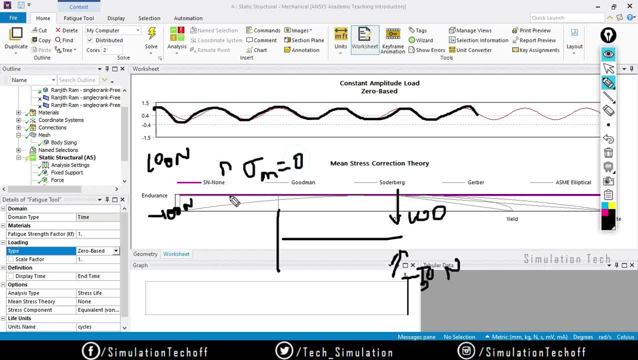 this mean stress, stress mean. so that is zero. So these two values is actually, I mean, equal. So that is why we are getting a mean value like zero. So in zero based, the load is actually look like this, the curve also look like this, So it does not get back up. 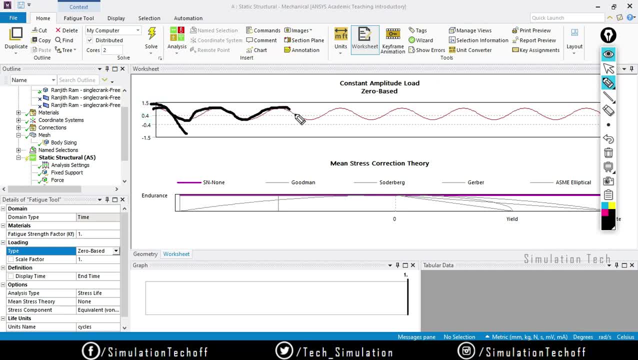 to here. So it reversed here itself. That is zero based. And also you have an another option that is called ratio. we can give the ratio. So right now it is taking the value that is minus one. it is a fully reversed condition one. 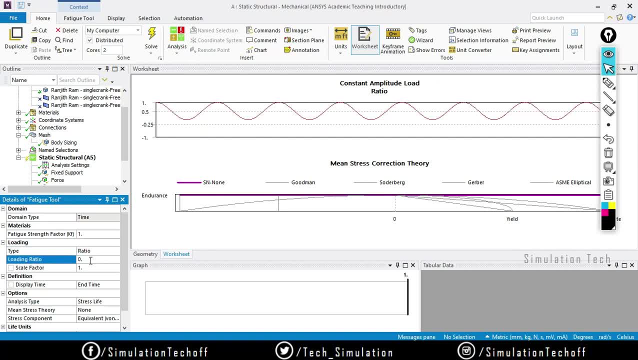 from here to here. So if I give the value that is zero, it is zero based one. So based upon the ratio, the value can be changed, the amplitude can be changed. But suppose in, sometimes I don't want these kinds of I don't want to give the ratio, or else either I don't want 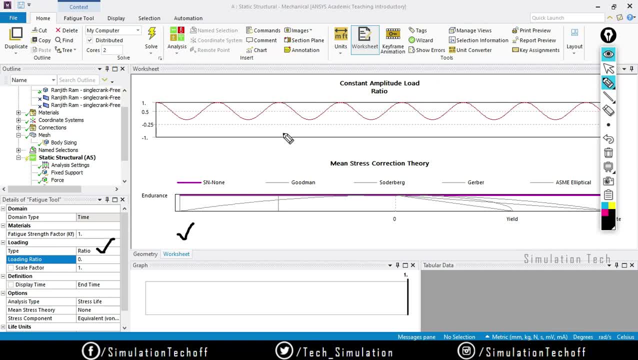 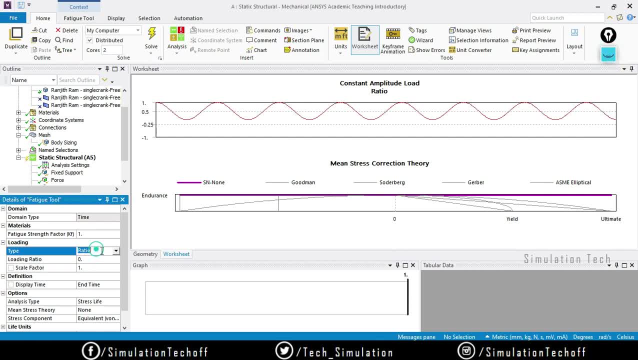 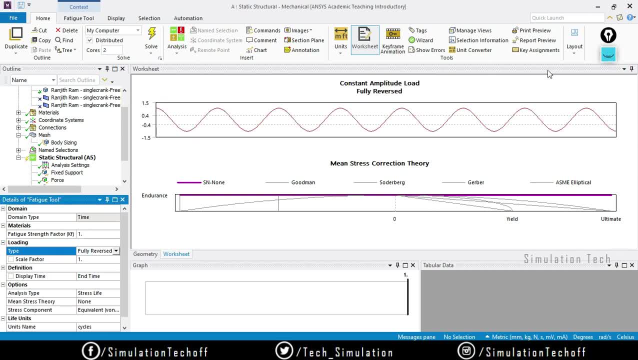 location. I'm choosing fully reversed condition one, And we will discuss about the scale factor here. you have an option called a scale factor. we'll see what is that scale factor in a couple of minutes after And when I go to that- these options- you have a stress life approach And 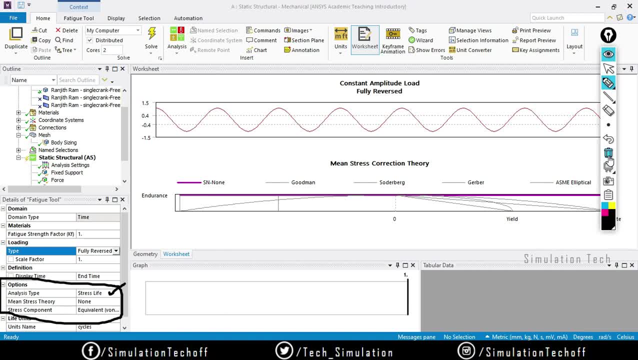 mean stress theories and stress components will explain one by one What does it mean. Like I said before, we have two approaches to solve this problem. One is stress life approach, Another onus strain life approach. you can choose anything And you know that. 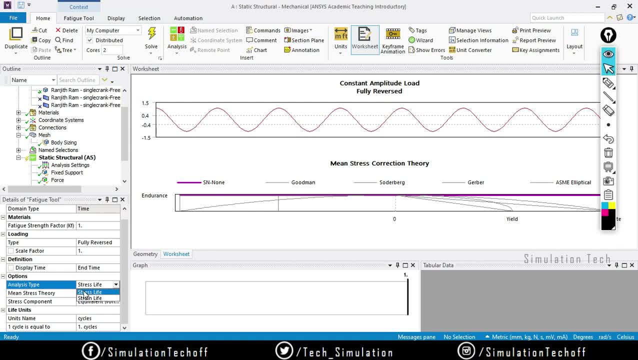 when to choose and why to choose that. So right now, I am choosing stress life approaches And mean stress theories. what is that mean stress theory? In this case, it is a fully reversed one, right? So we are having this bar, So these 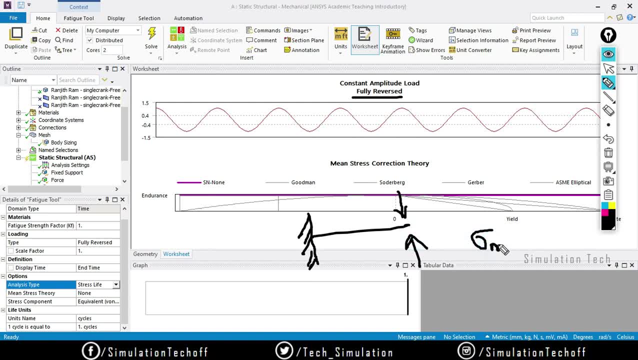 load is 100. And these load is under the mean, is stress minus zero. But in real time there is no such situation like that. So every time, so when you apply a load, the reverse load cannot be the same load. So we are having a. 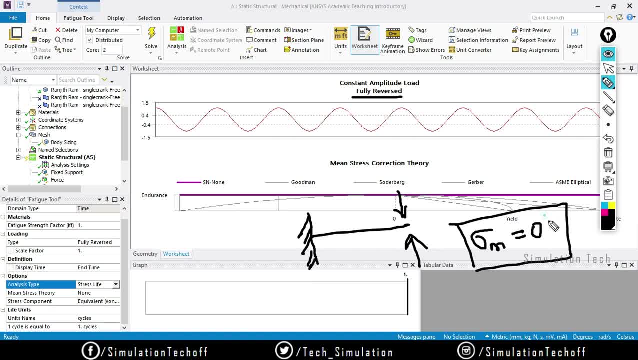 actually some values there. So to rectify this error we have this mean correction theory, So that is called mean stress correction theory. Basically we have a four methods to correct that value. That is a good man, Soderbergh, Gerber, And also. we have another method also. 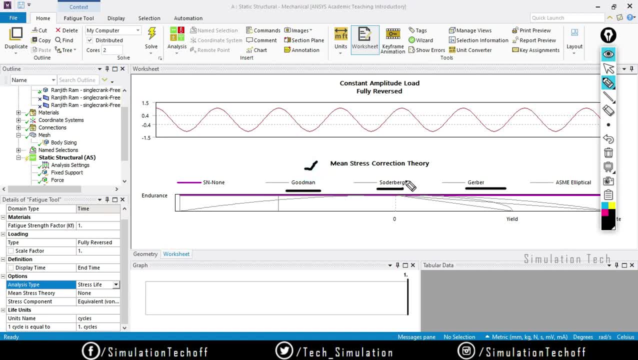 And hope you already studied this methods in your strength of material subjects. I hope you will use this. So we are going to start with non-standard theory And we are going to start with non-standard theory. So first of all, we can go to onglyph theory, Which is 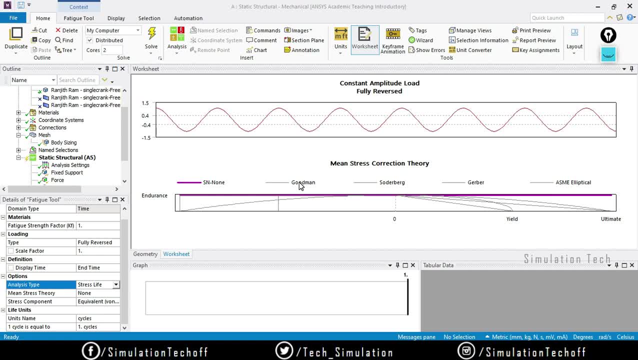 a very simple theory that is a little bit complicated to study. It is a very simple one. So if you have a good man- Soderbergh, Gerberh, Gerberh- and know this theory, you can use Gerberh theory as a theory and you can estimate the theory of a man If you know. 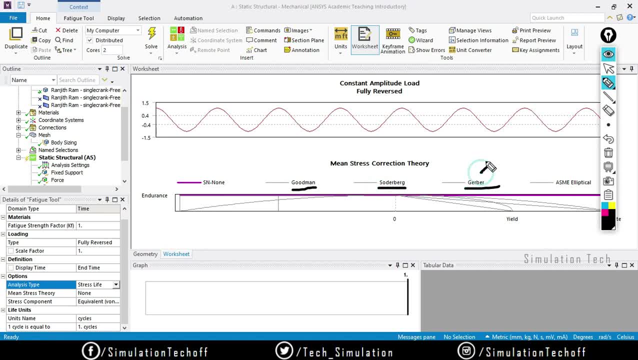 this theory. you must study each and every theory separately. It has a lot, a lot of calculations and theories itself, But we have certain recommendations: when to use good man and when to use Soderbergh and when to use Gerberh. GERBERH Theorist. for most of the ductile material like aluminum or copper, you can use Gerberh. 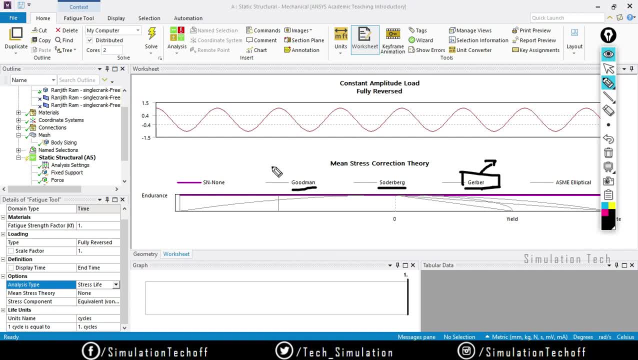 But for a brittle material like steel, cast iron, like that, you can go for Goodman. It will give you the better result, But it's actually not like that. But you have to use- I mean study about the theories and you can choose. 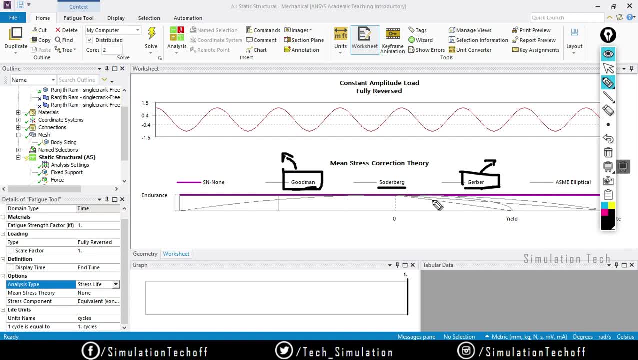 So in which time I can use I can go for Goodman theory and which time I can go for Zerba theory. So right now I'm choosing Goodman. And also you know about that- equal and one Moises. equal and one Moises means this is: 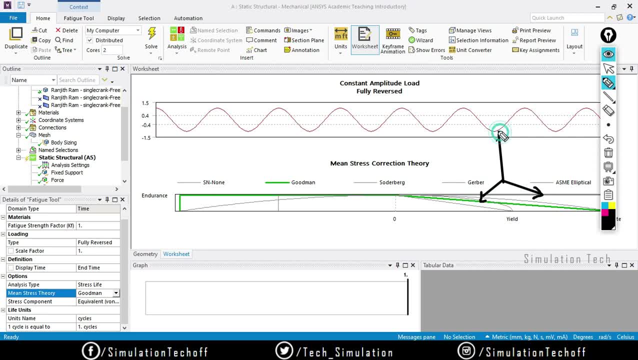 my coordinate system. So whenever your component is experiencing the stresses in different directions, like x axis, y axis and z axis, you have to combine that into a single value So you can use a one Moises stress So like also. But in that normal static section you have only one method that is equal and one Moises. 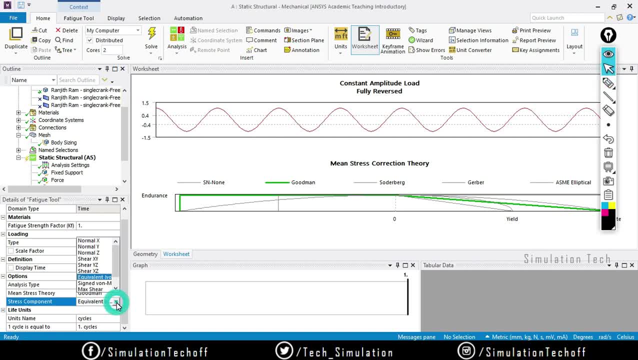 Here we have a different method to combine the stresses. That is equal and one Moises signed, one Moises maximum shear and maximum principal and absolute maximum principal stresses And also this is shear on x, y and y, z and x- z. 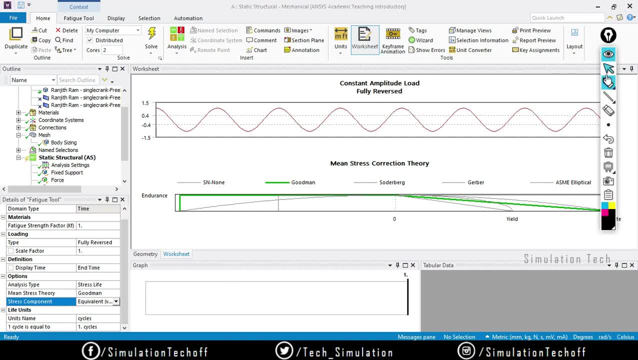 Here also some recommendations are that when to use that For a brittle material, you can go for signed one Moises. if it is a ductile material, you can go for ABS. that is absolute maximum principle. it will give you a better results. 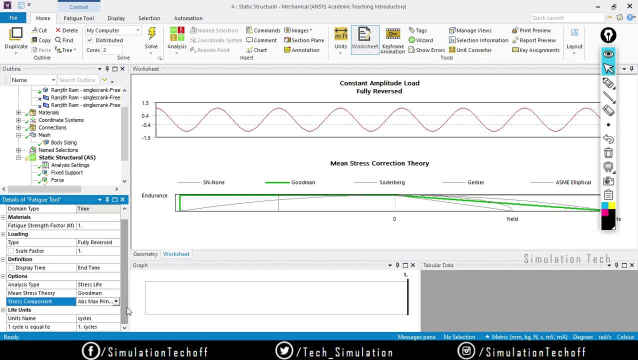 So I will choose any one that is absolute maximum, principal stresses. And also you have that lifetimes, in which units you need that lifetime, whether it is in cycles Or seconds, minutes, hours, days, months, you can choose. So I am choosing cycles. 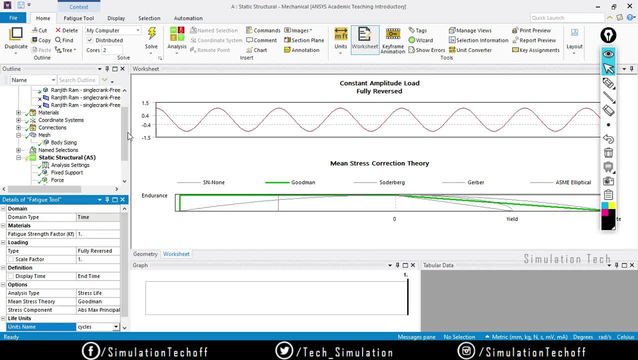 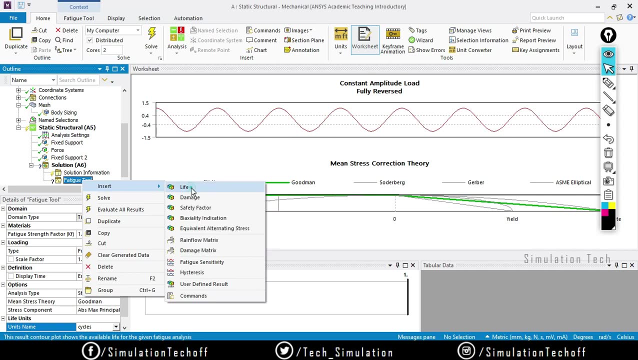 Okay, So that is all for this, And when you want, so still, we have that question mark Here, we have the question mark over here. So I- because we don't add anything in the fatigue tool, so right click and insert. So I want life and right click, insert, I want damage. 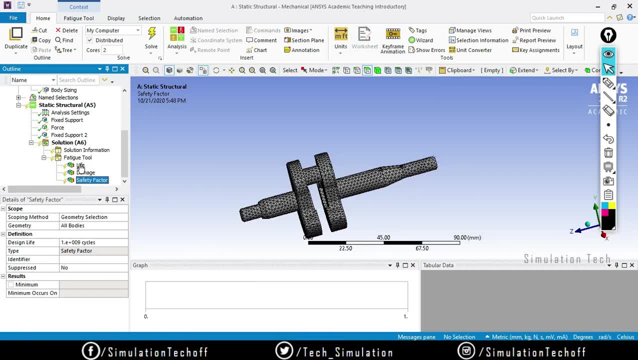 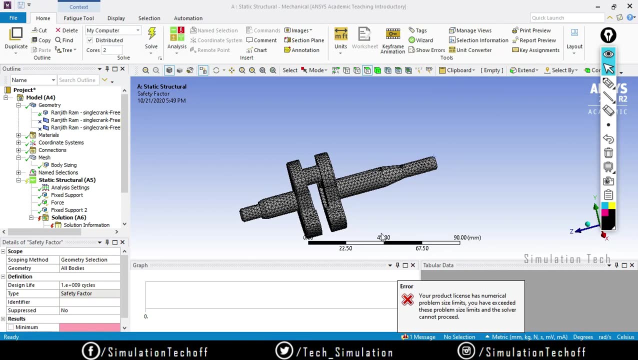 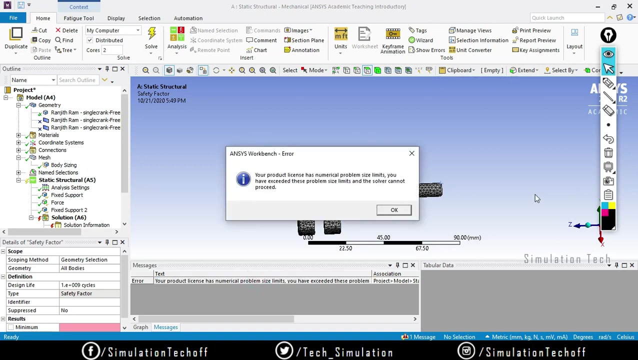 Now also right click insert. I want factor of safety. So life damage and factor of safety. So once you click on solve, I will minimize it. Okay, so we have excited. I mean your product license has a numerical problem: size limit. 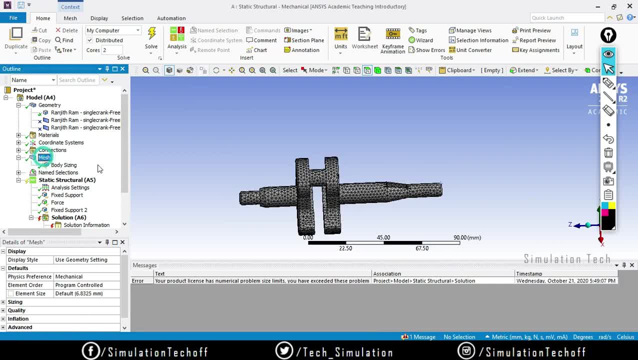 Okay, fine, Okay, Okay, Okay, I will check my mesh data. Actually, it doesn't do it. then, Okay, the notes. So the allowable limit is 32k, But right now we have around 50k. So what are you going to do here? is I just reduce that set? 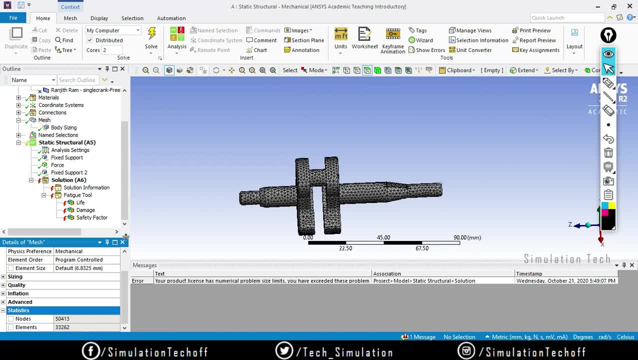 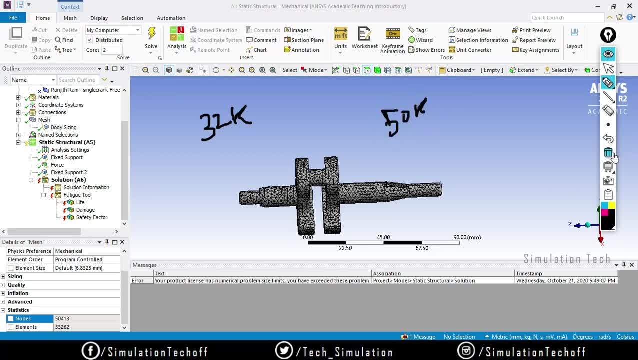 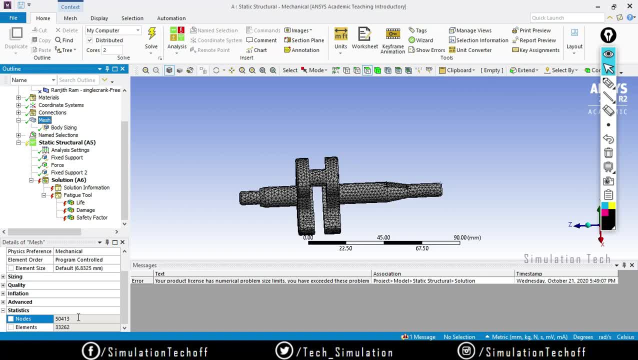 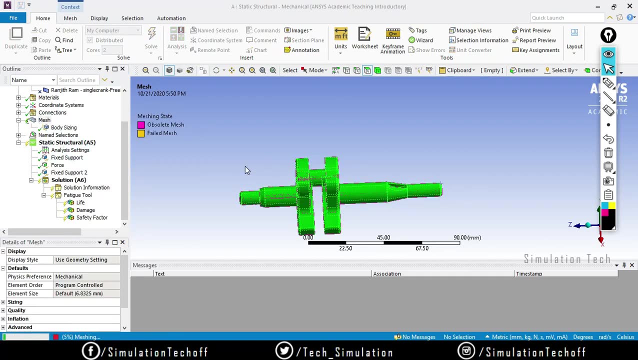 It's not Okay. Okay, So in normal, correct version you can create any message So we'll reduce the cipher- I mean size factor, that is, two mm to four mm, And rightly can say generate mesh. Okay, let's look to maybe three mm. 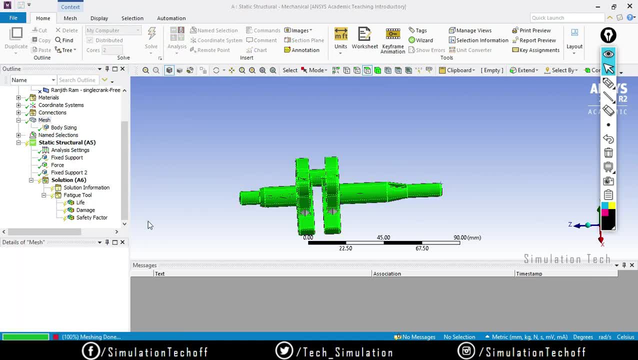 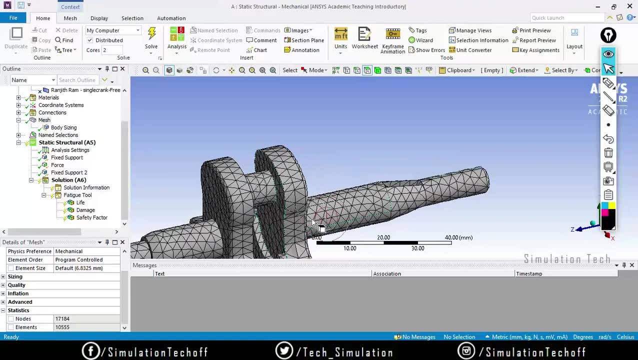 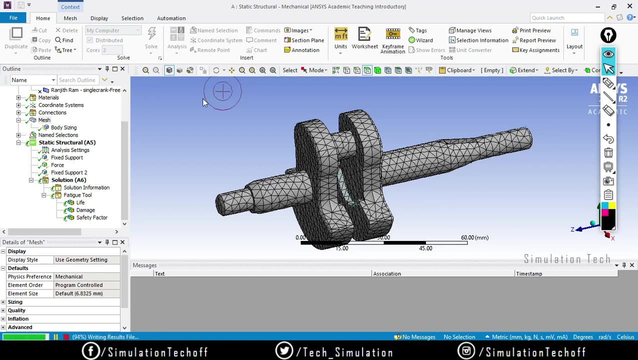 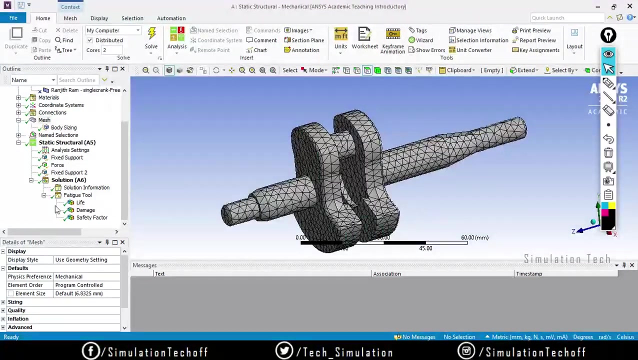 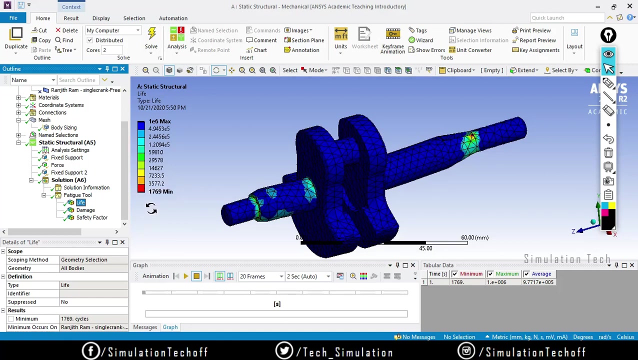 Okay, find much better. okay, good, so still now it's a poor mesh, but it's okay. click on solve: okay, now our problem is get solved. so when I click on life, you may have a value from 1, 7, 6, 9. that is your minimum cycle, that is it actually fails is over. 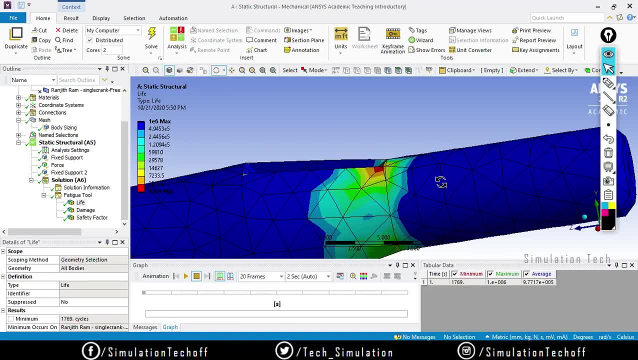 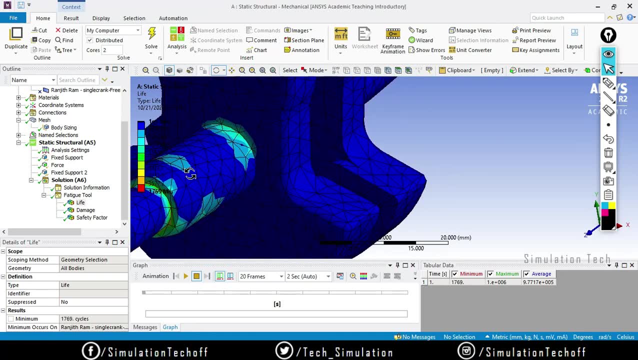 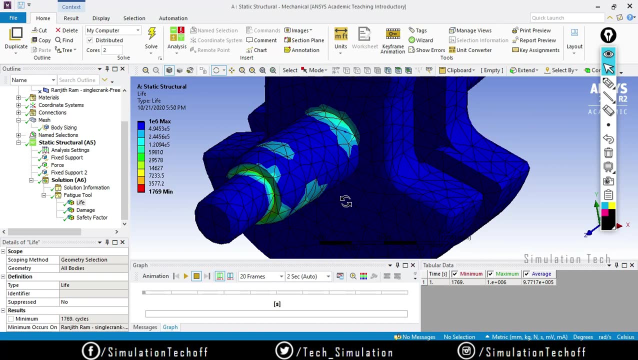 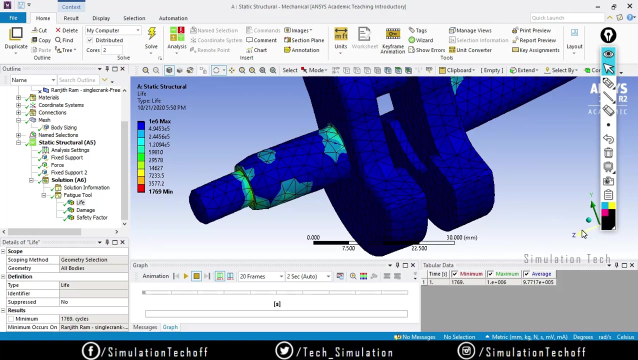 here because we are applying a fixed support over here. what does it mean? start cylindrical support? a cylindrical support means only the rotations will be free. the all the translation is actually locked- rotation about these axis, like this perpendicular axis, right now it is Z. the rotation about Z axis is actually free. it can be rotate. 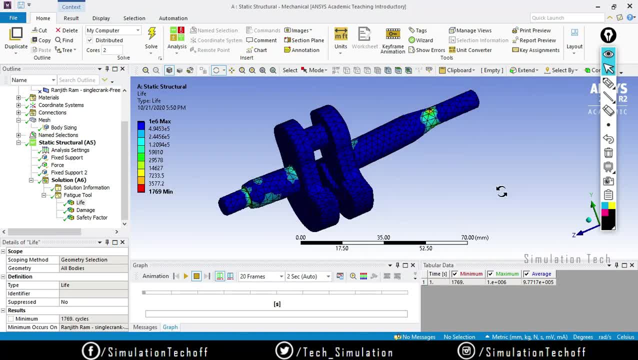 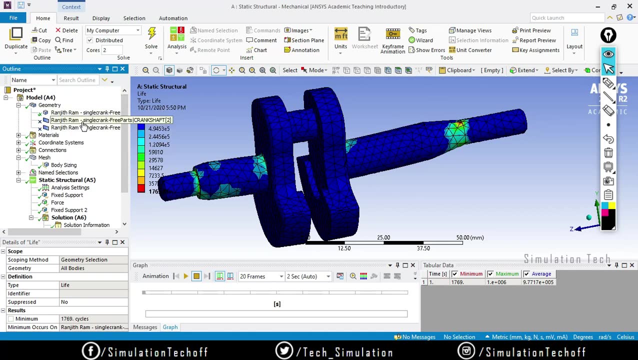 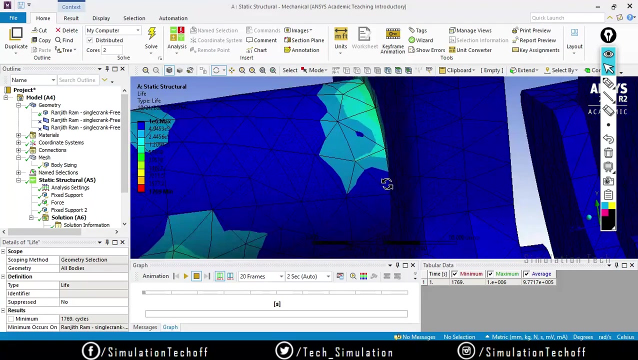 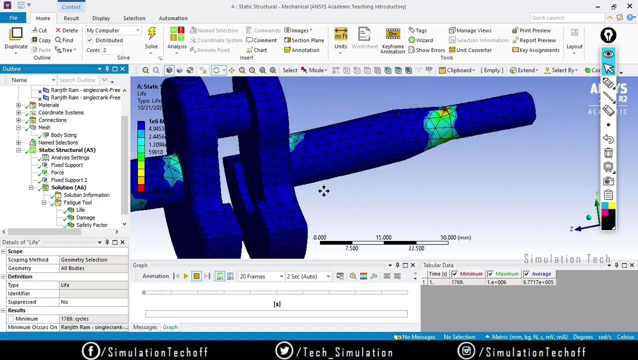 anywhere, and also it can be moved about in Z axis itself, but not in Y or X axis. so that is called cylindrical support, so you can unsuppress these two things and you can use the surfaces to assign the cylindrical support also then. so actually the failure is happened in this region, so it only lasts. 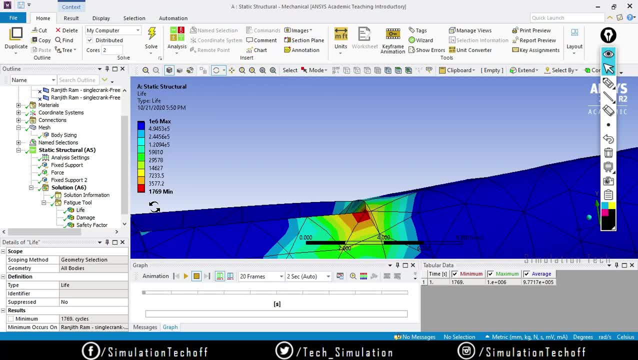 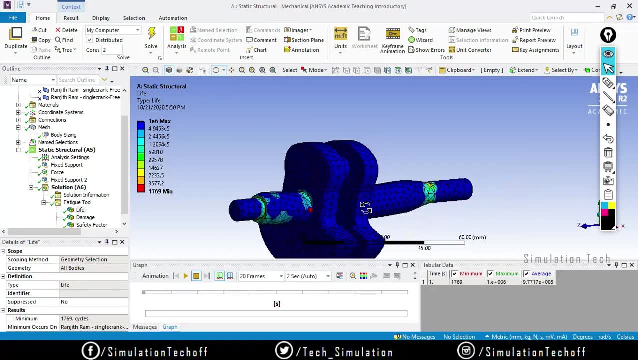 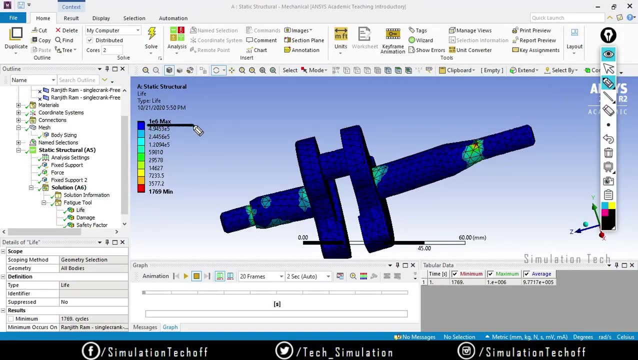 for thousand seven hundred and sixty-nine cycles. the remaining area is fine, and whenever you get a value like this, like 1 e, power 6 is gone. But once you get an agreements value, it's quite easy. so for both minimum and maximum, so your component having an infinite number of. 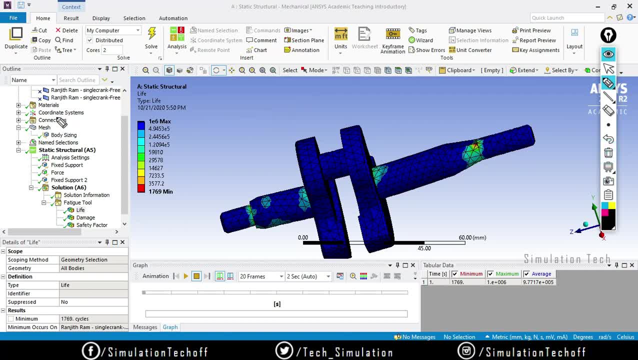 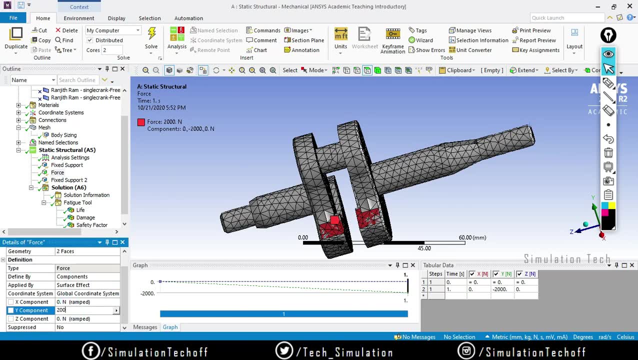 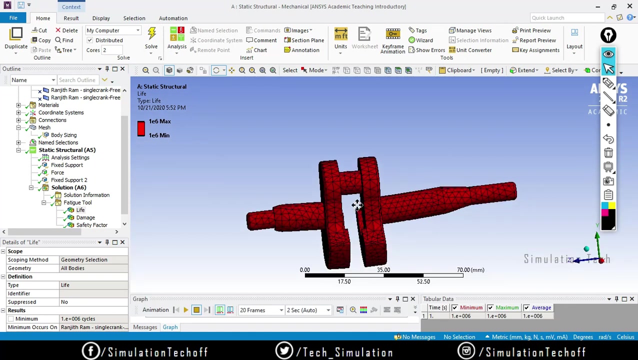 cycles. so you can assume that. so when I try to reduce that, we will click on to the force and reduce the force to 200 Newton minus 200 and click on solve. see? so just because it looks like some red color it doesn't mean your component is failed. so its color is just for the aesthetic appearance it shows. 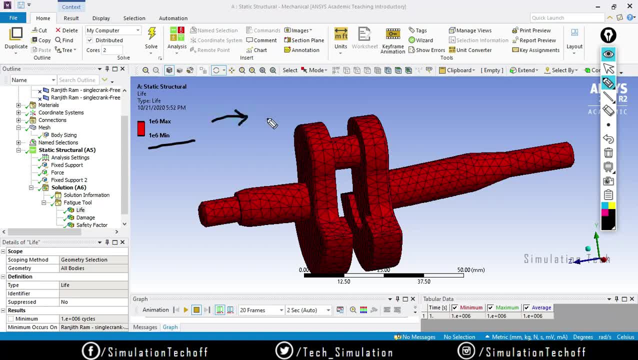 the value that 1 e power 6. that means your component has infinite number of life. there is no damage for this type of load, so it can last for 1 e power 6 cycles. okay, and I click on that damage. choose that thousand. there is no damage at all. 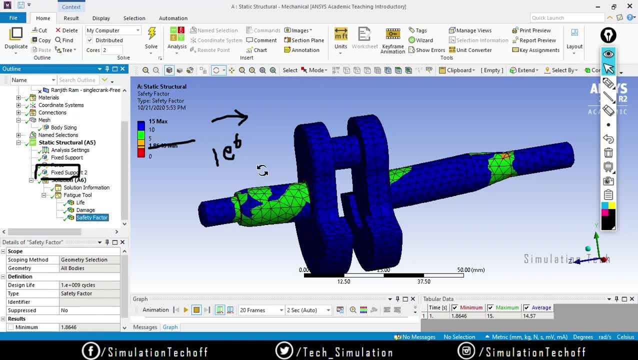 because the load is very, very minimum. and factor of safety. the factor of safety is: if you are having more than one, that is fine, you don't have to worry about that. you don't have to worry about that. so yeah, in our theory decision I say that when you get the value, 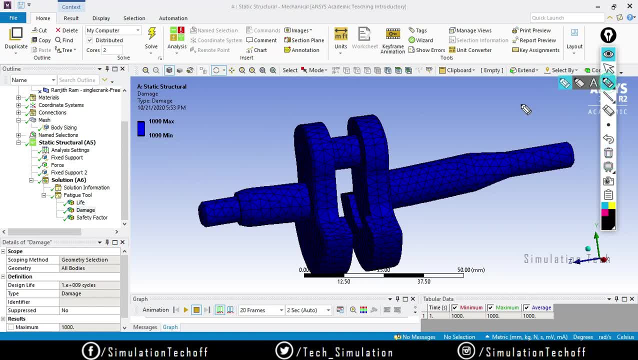 which is more than one. your component is surely failed, But right now it shows that 1000.. But I, but my component is not failed, how it is actually looks like, So how I actually says, okay, it is not failed, But right now. 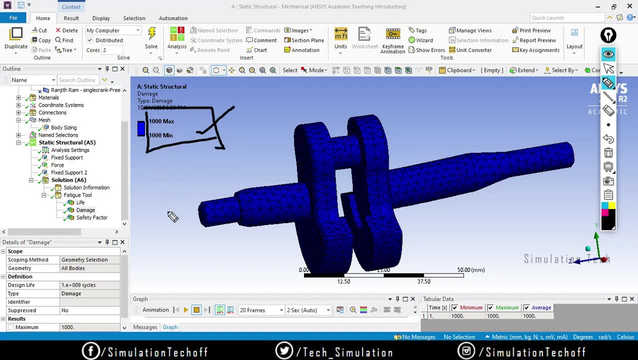 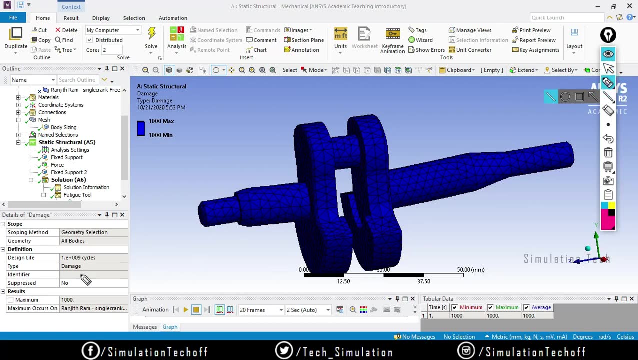 instead of showing me a one, it shows the value called 1000. So actually it depends upon these value. here, in the detailed review of the damage, you will notice that there is a factor called design life. In design life itself it says that I need. so my requirement. 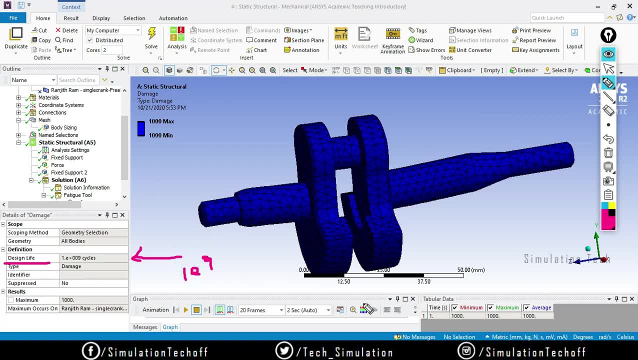 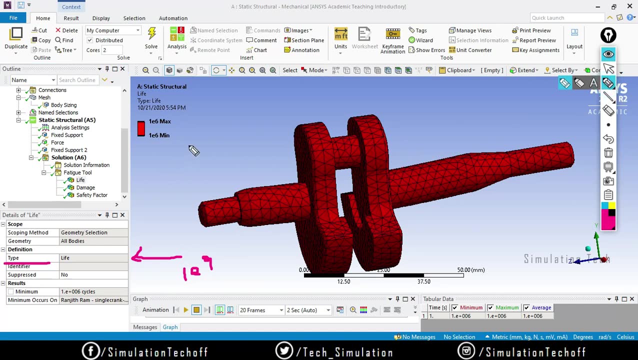 this is my requirement. one e power nine. Okay, But right now the component life is. when I click on life, it shows that my component life is one e power six. So balance: we have 1000.. So that is why it shows it says that 1000.. But if I reduce that value, 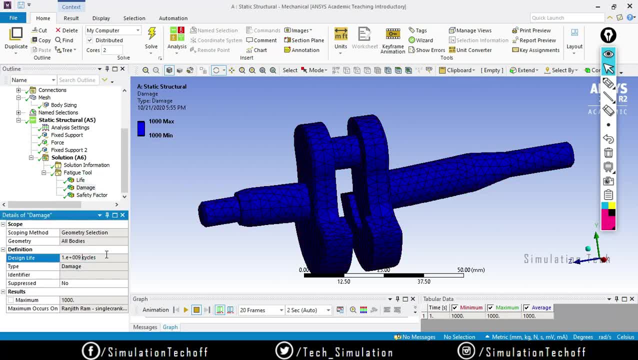 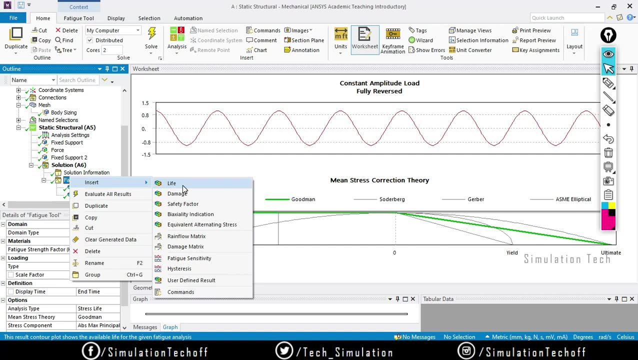 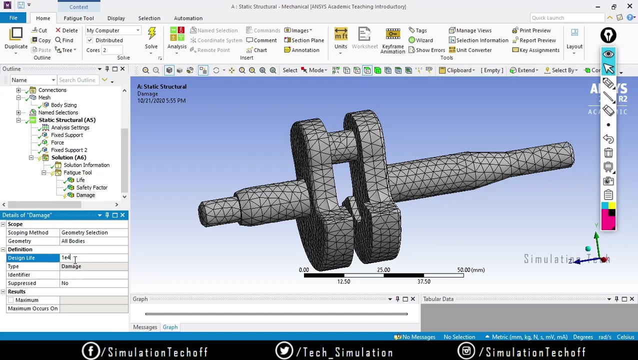 reduce the value damage and click on it. I'm reducing that to one e power five. Okay, Right now I can't edit, just delete that And insert another. damage Now set the value. that is one e power four. So this is my actual need. So I want a component should be sustained for one e. 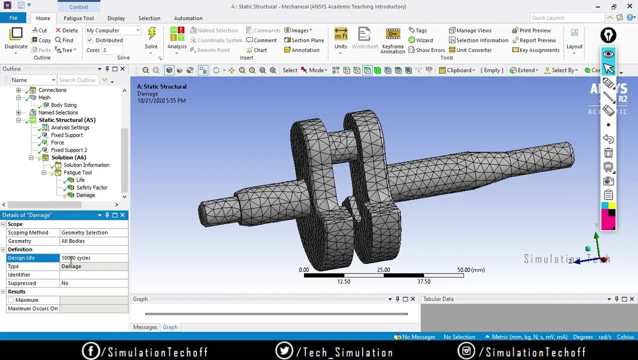 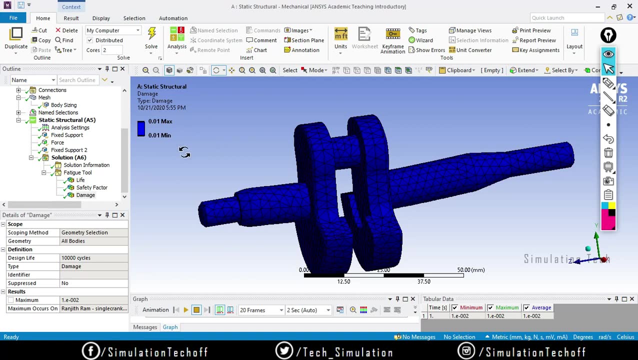 power four cycles. Okay, that is a 10,000 cycles, I mean not 10,000.. Yes, 10,000 on e power four And click on solve. So this time you will get a value which is less than one. So it depends upon the factor you. 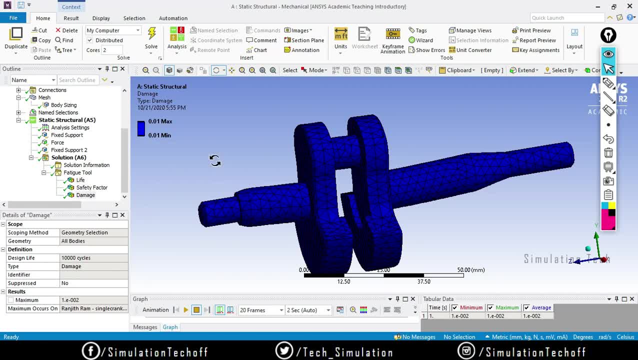 entered here. If you are getting a value which is lower than one, your component is not damaged. For factor of safety, you have to. the value should be more than zero. I mean more than one, not zero. If you are getting the value less than one, your component is failed. So let us increase the. 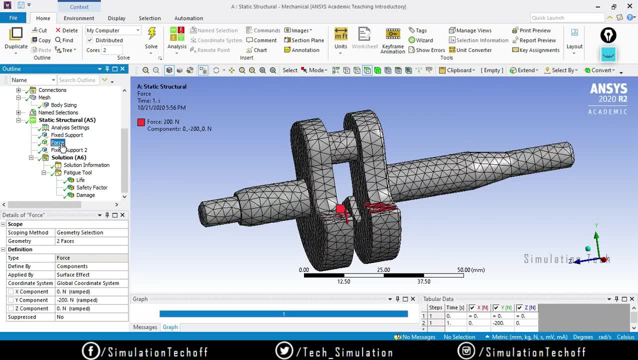 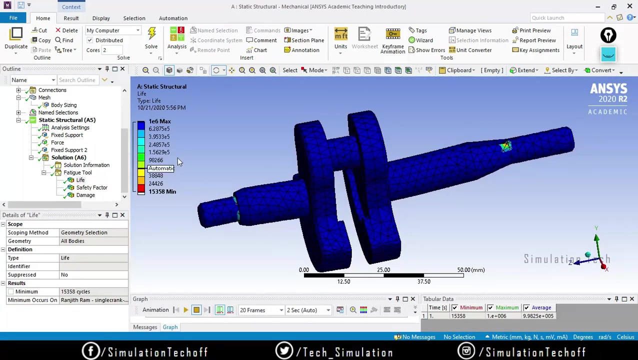 load factor to. I mean 2000 to 5000, 5000, not I mean 200 to 1000.. What happened and click on solve. Okay, now I click on solve, I mean life. I have a maximum life. my failure is actually happened in. 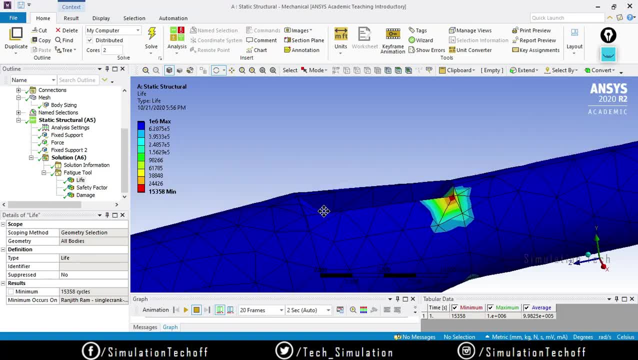 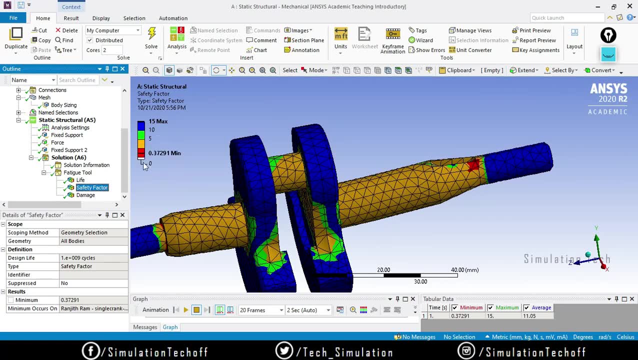 this region. Okay, now I click on solve. I mean life. I have a maximum life. my failure is actually happened in this region. That is a last five, 15,358 cycles about factor of safety. it is less than one, so surely my 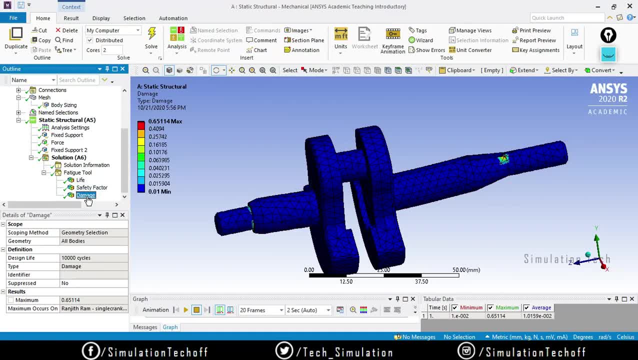 component will fail and damages also- Okay, damages four k, which is less than one, but my requirement is very low. So if I try to increase my design life, so obviously it will be failed. So if I try to increase my design life, so obviously it will be failed. Also, you have an option in fatigue tool that is 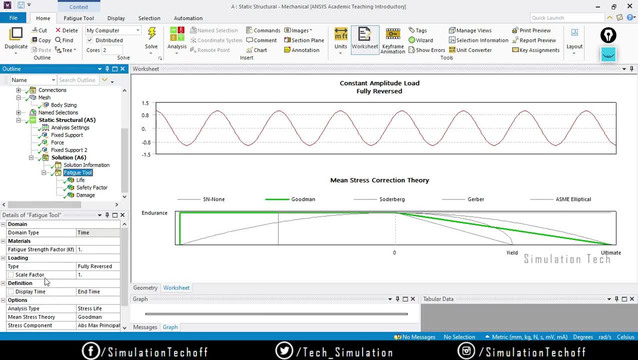 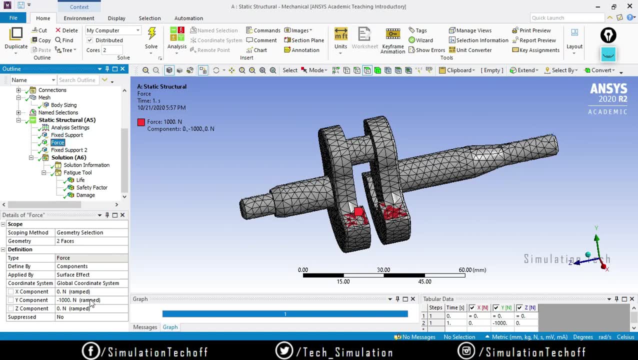 Also, you have an option in fatigue tool, that is tool, that is scaling factor. suppose you don't want to increase the load. so right now we don't, we have only one load, so that is why i'm go and increases the load. suppose you have a lot, a lot of loads like here you have a load and here you have a load, another load. 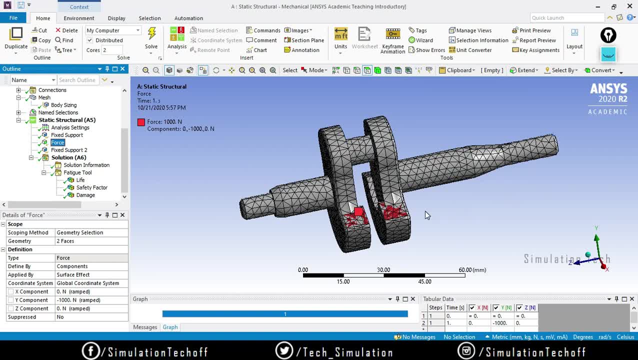 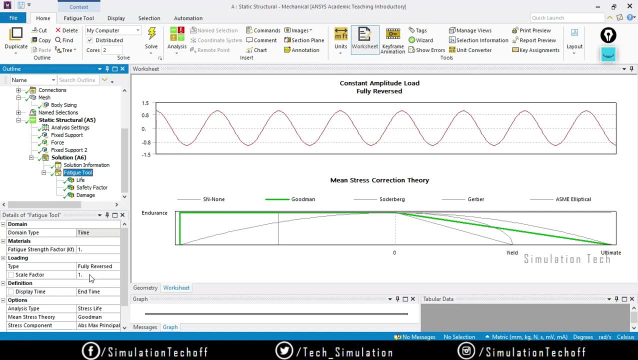 10 to 20 loads you don't actually increases the load factor one by one. so for that you have a scaling factor, whatever the scaling factor you give over here or assigned over here, so that will be reflected on here. i mean, suppose i want to scale my loads into three. 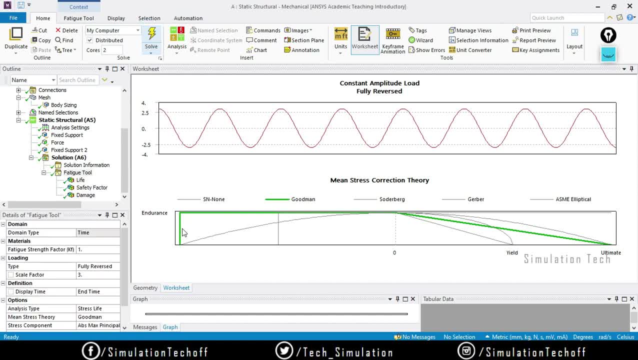 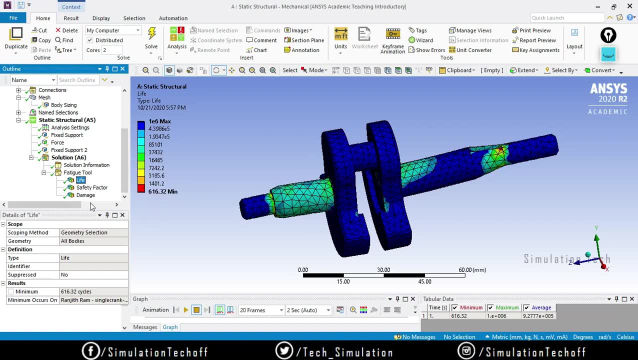 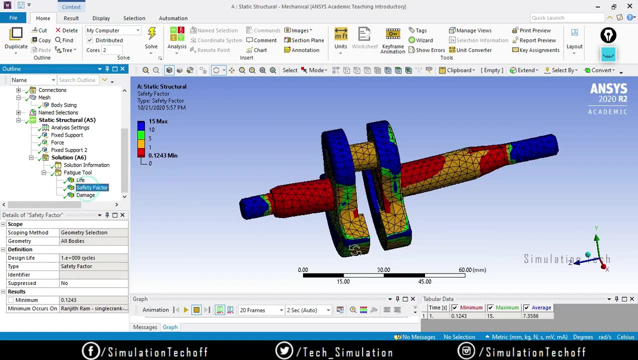 times, three times, and click on solve, so it will be get solved. now the life is furtherly reduced because my load is actually scaled three times. factor of safety, you get a very low value and damage. also. you can also animate it. so if you're on the animation, you can animate.